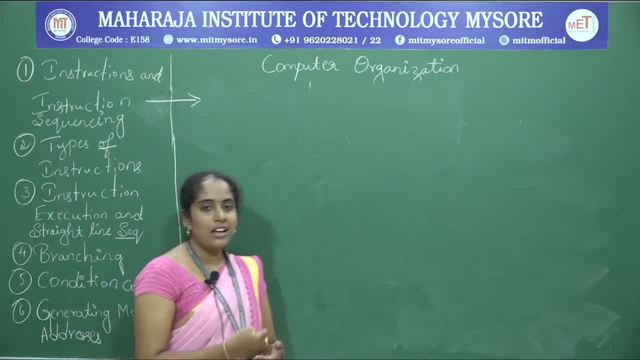 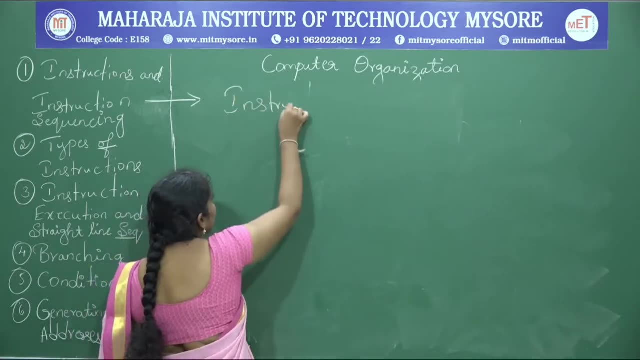 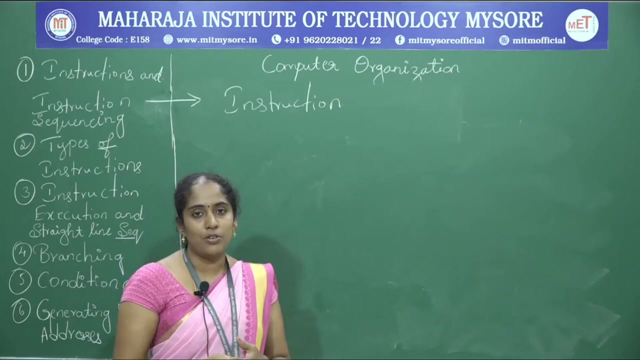 program that will be stored in the memory. So here the program is nothing but the instructions, machine instructions. Okay, so here, to perform any task in the computer it needs some set of instructions that is already be stored in the memory. Okay, so that set of instruction will be stored in the memory. 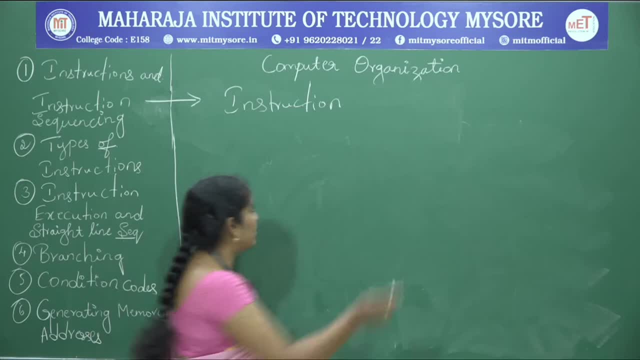 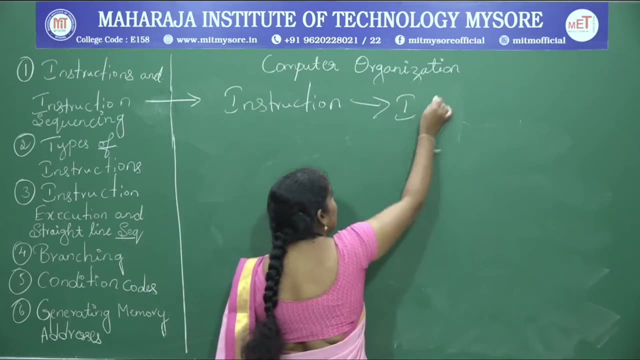 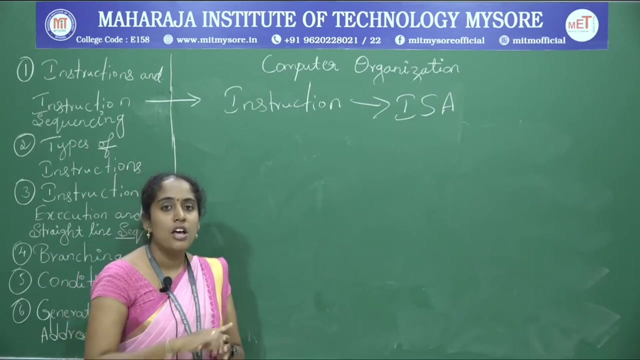 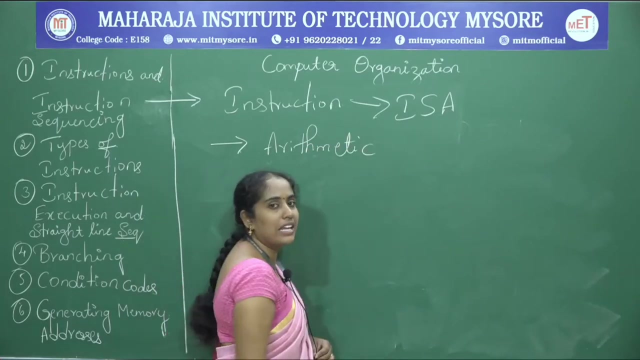 So that is called as instructions set architecture. So set of instruction group. that set of instruction is called as instructions set architecture. Here computer will perform the four types of operations. Usually it performs four types of operation. in that first one it is a arithmetic and logic operations- Arithmetic. 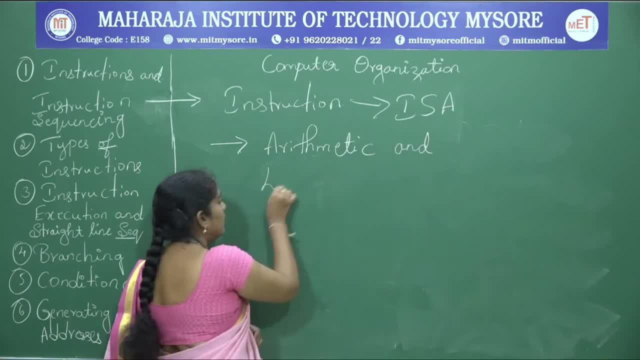 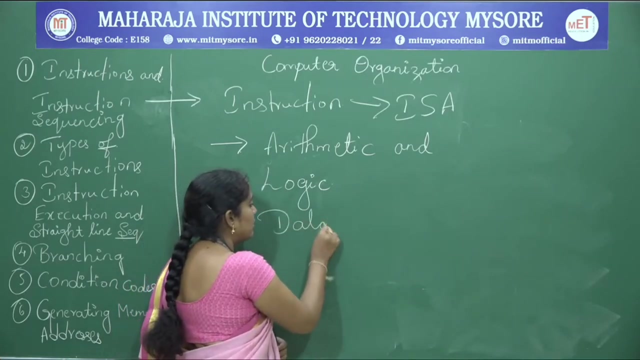 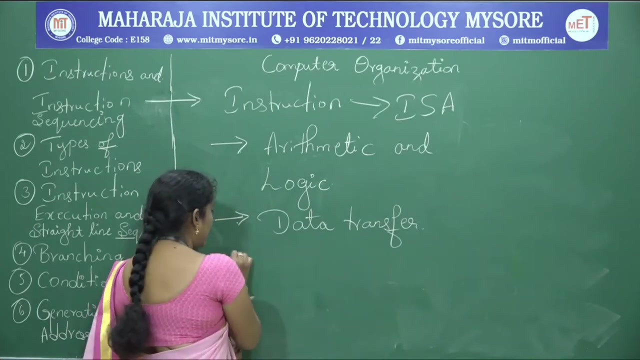 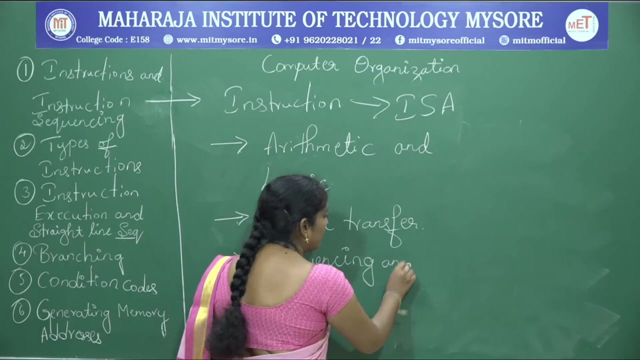 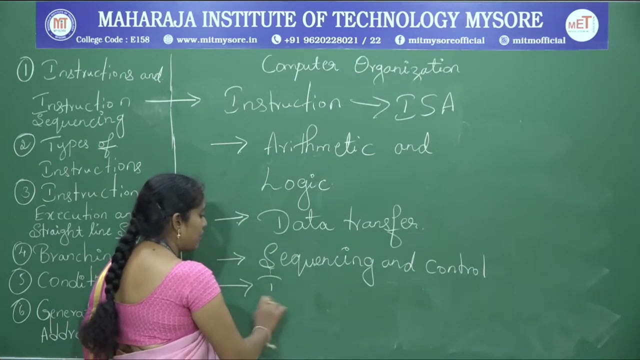 and arithmetic and logic operation. and second one it is a data transferred between the memory and the processor. that is a second task, So data transfer. and the third one it is sequencing, program sequencing and the controlling. And the next one it is inputs, output operations. So it does perform these operations, the computer. 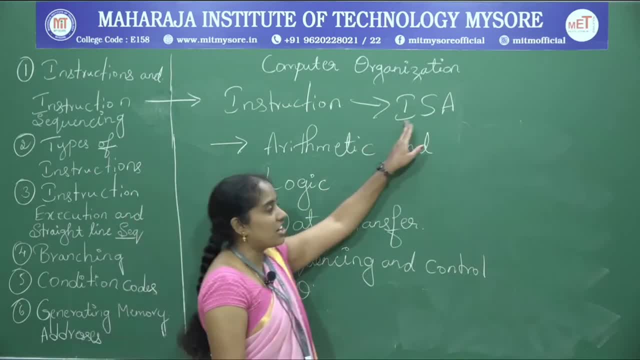 will need the set of instructions or instruction set architecture. So in this instruction sets that architecture, in this instruc- Technical timed Aquatic programming program using which toV AO sending mller and output operations five depends on this Doctors. So this application, shape it and this function. 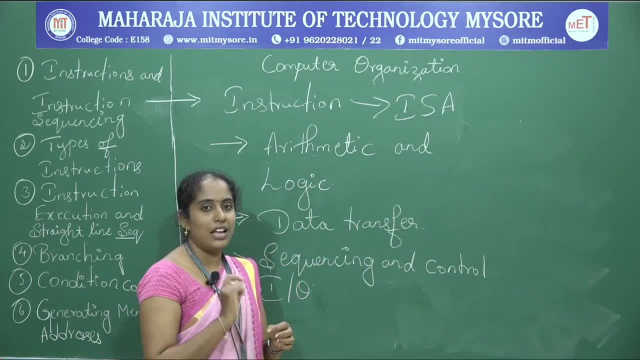 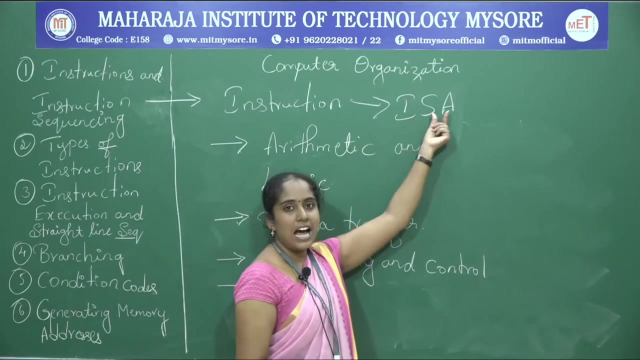 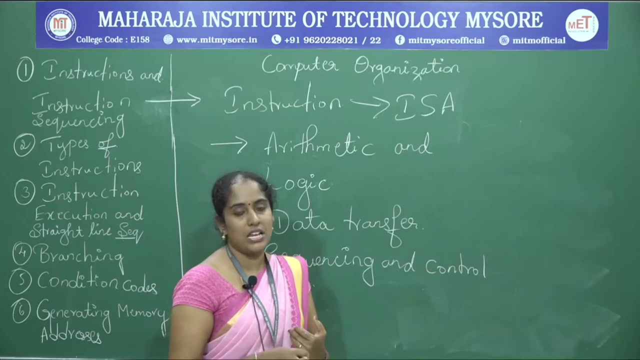 instruction set architecture how your computer will understand the. so it needs instruction set architecture. so how in this instruction set architecture the operation and operand will be represented. so in that we have two notations. we are using two notations in that first one is a register transfer notation and second one is the assembly language notation. 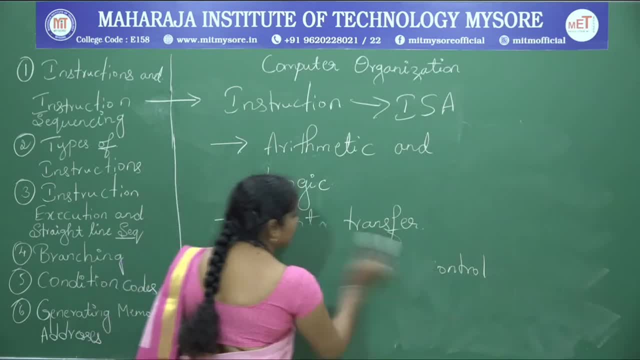 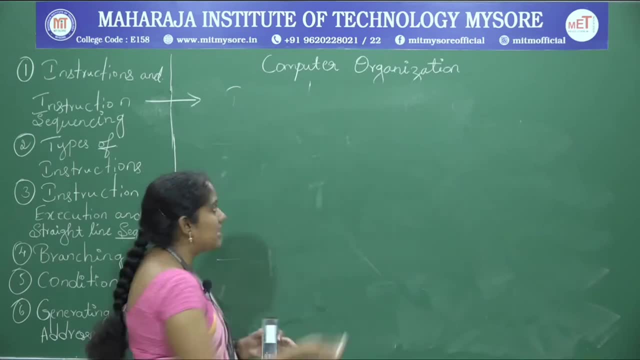 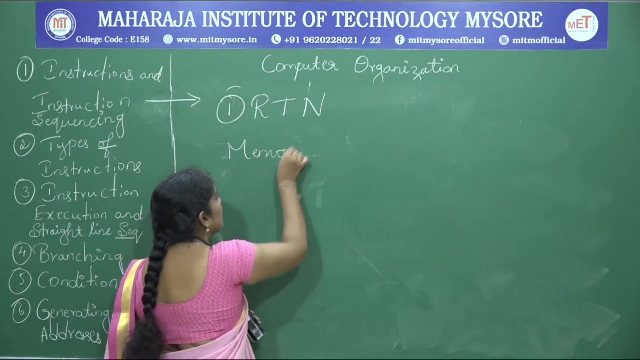 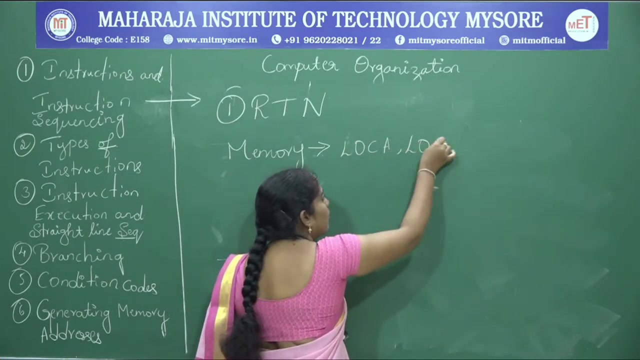 so first we see register transfer notation. first one is register transfer notation. ok, so in this, in this, the memory location name will be represented as capital letters. so memory will be represented as like location A, LOC A, LOC B, LOC C and all, or else A, B, etc. ok, so next. next the 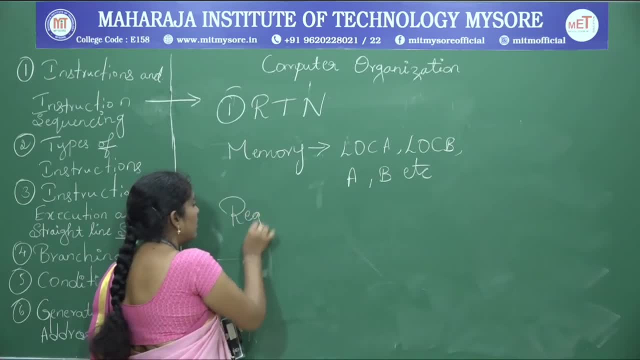 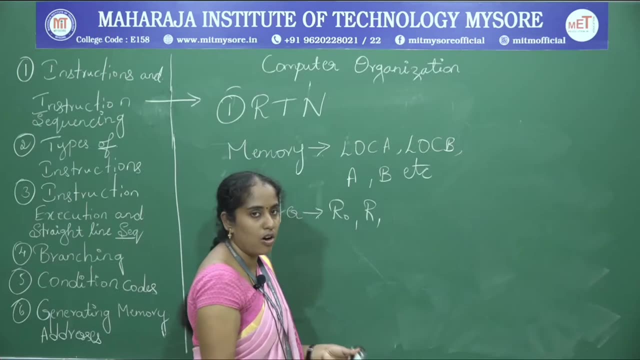 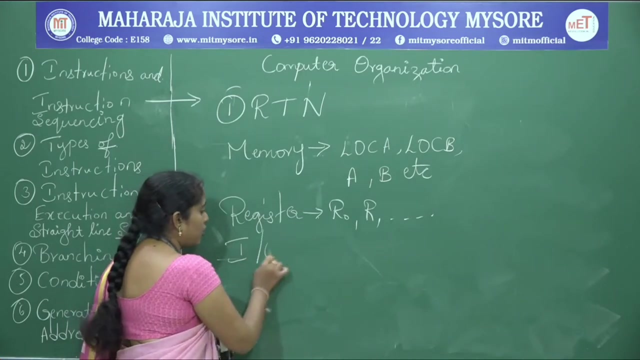 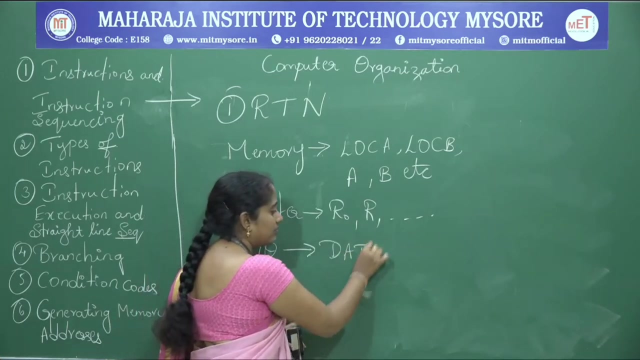 processor registers. registers will be represented as R0, R1,, R2 and so on. ok, so next it is a input output: input output operations. in the input output operations it will be. it will be represented as, like, data in data out and the out buffer in buffer, like that. 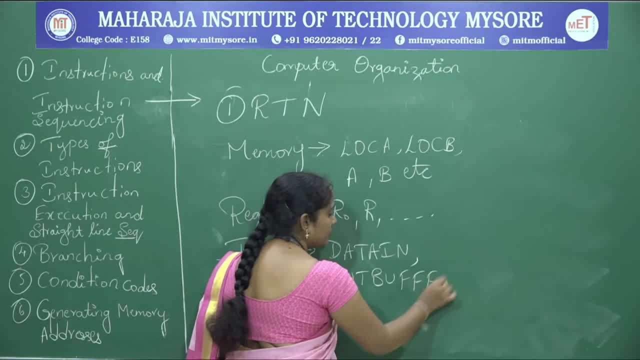 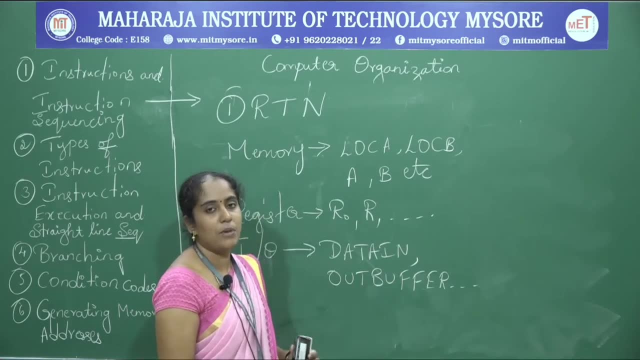 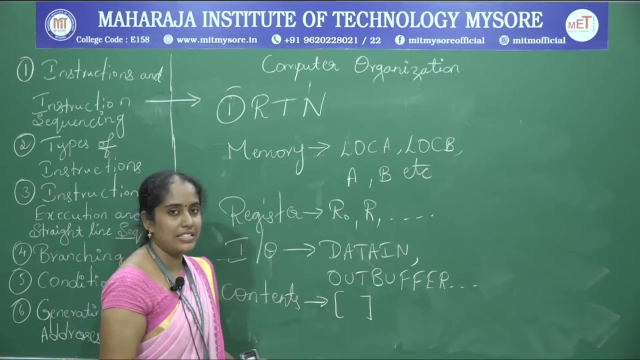 etc. ok, here to represent the content of the location or content of the register by using the square brackets. so how to represent the contents By using by using square brackets. ok, so here, after this, take an example: C is equal to A plus B. 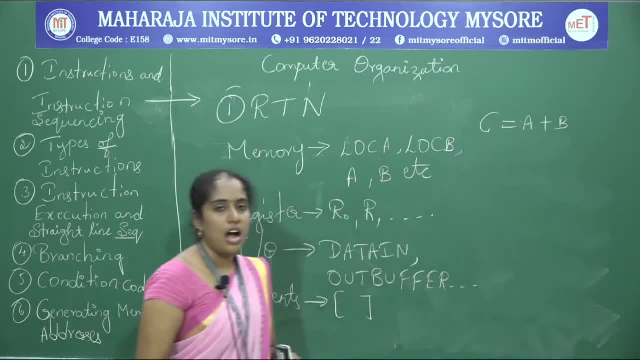 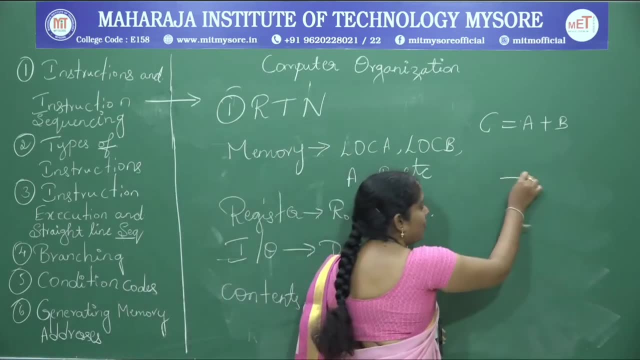 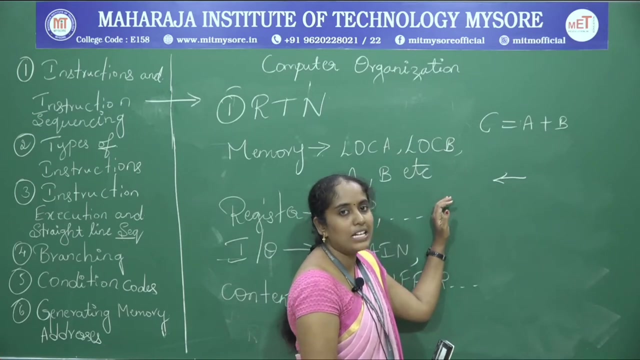 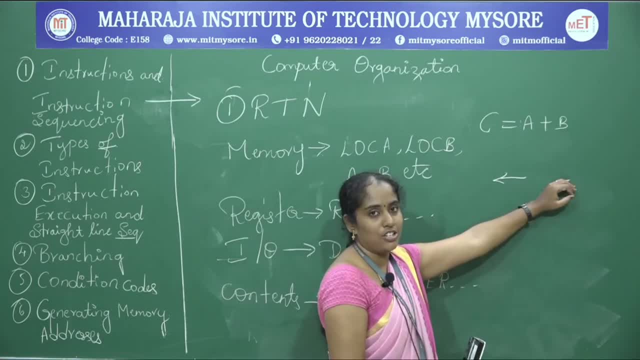 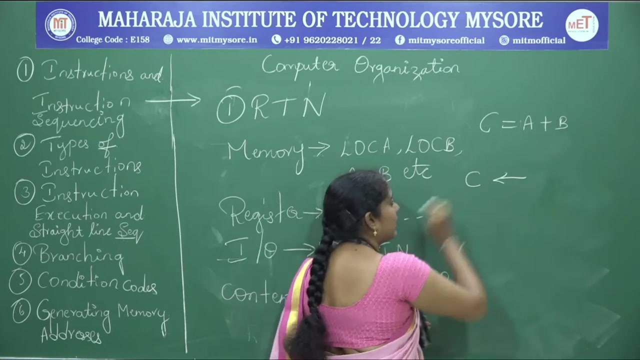 will contain the contain the memory location or source right. it can be memory location, it can be register, but the right side it will contain the source right. So here C is the destination and A plus B source right. so C, right side it will contain: 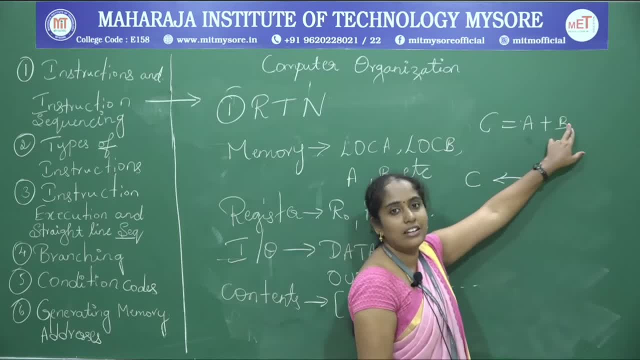 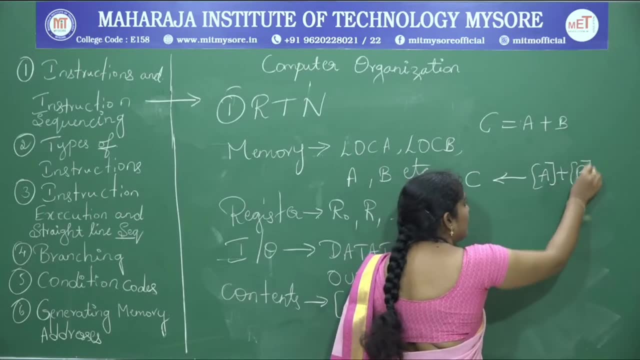 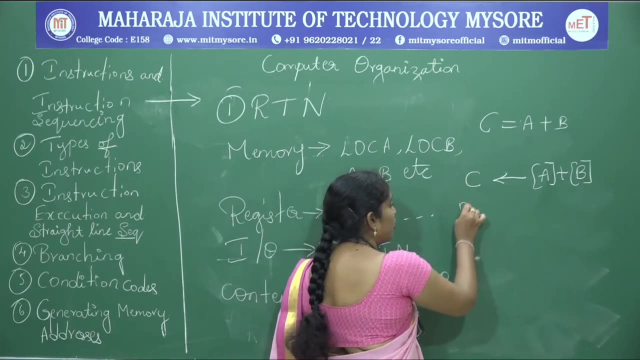 C. here you are adding the content of A with the content of B, right? so for that I am writing like this: A plus content of B, right? take another one example, right. say, for example: you want to move, you want to move the data from. you want to move the data from you want. 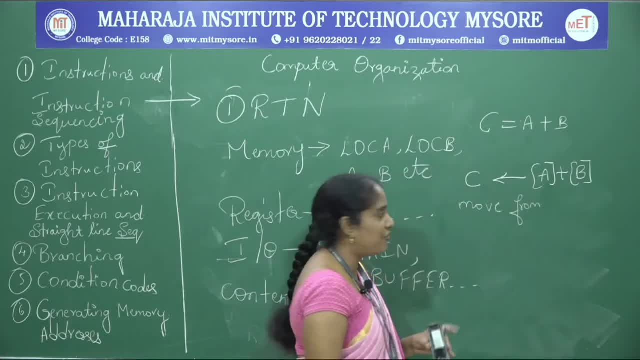 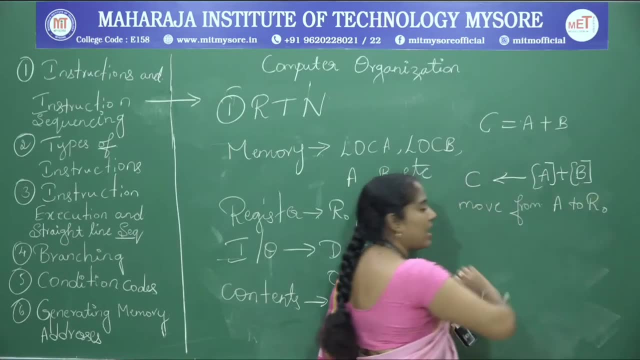 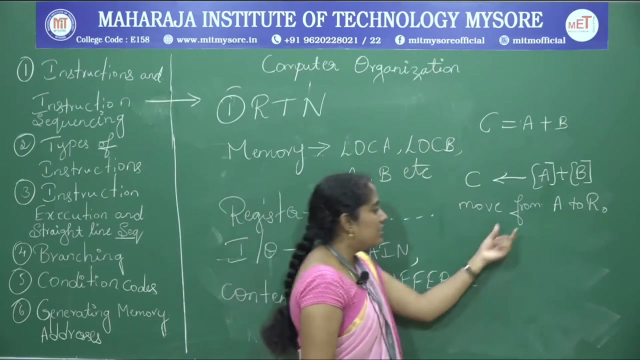 to move the data from, say, from A to A, to register R0, how to represent this A to R0 in register transfer notation. yes, here you need to find out. first you need to find out the destination. R0 is the destination right. 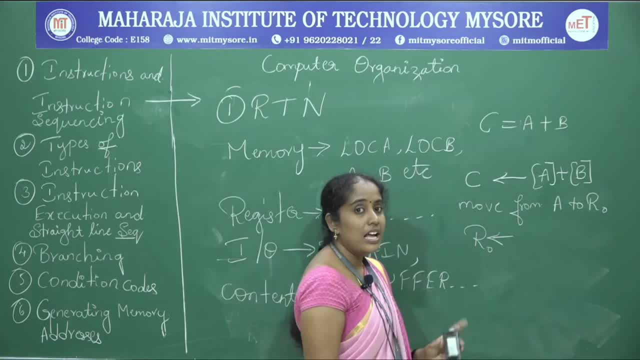 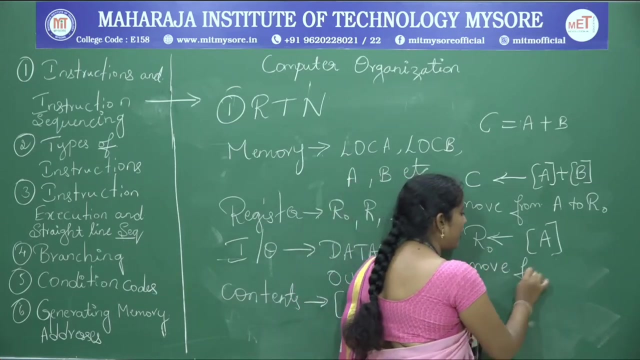 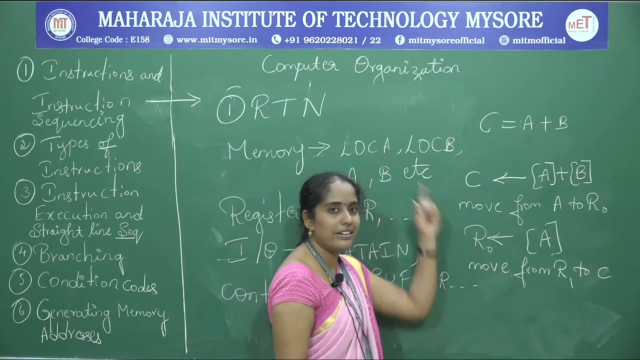 So for that right side it contains R0, right in the left side it is the source. so here A is the source, it is the content of A will be moved from A to R0, right, okay, can you write: move, move content from from R1 to C. how to represent this in register transfer? 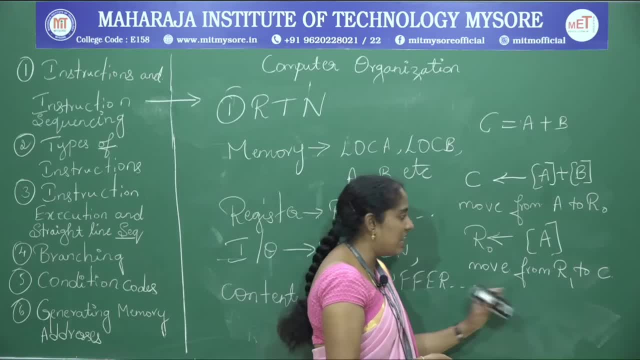 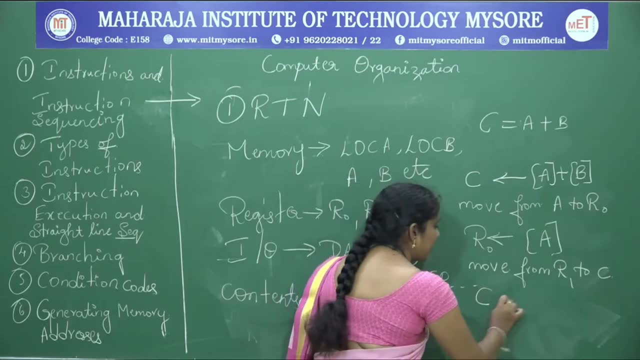 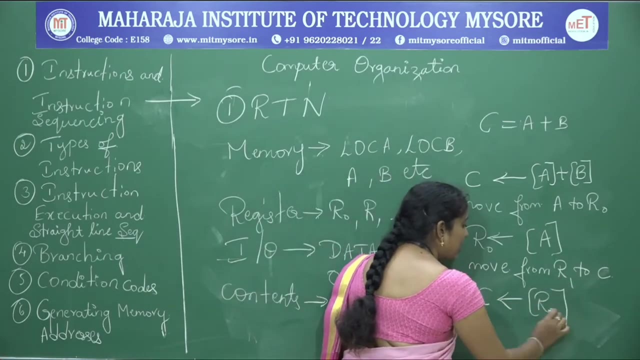 notation: yes, in the right side, sorry in the left side. first we take the source: sorry, destination right. so here C is the destination right C. So in the right side it contains source: here R1, so content of R1, content of R1 will copy. 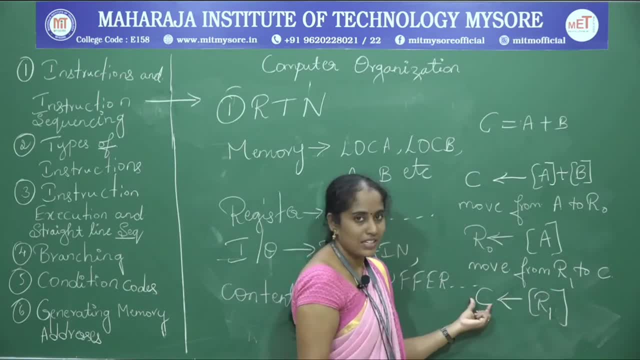 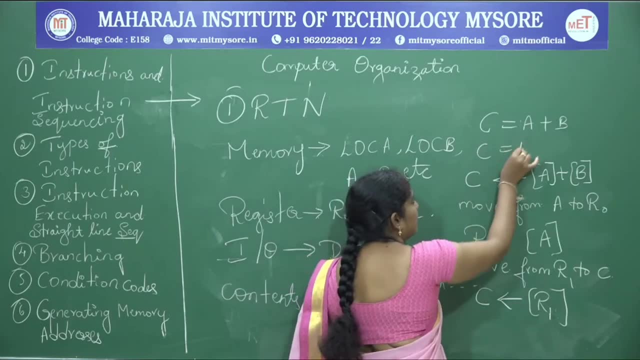 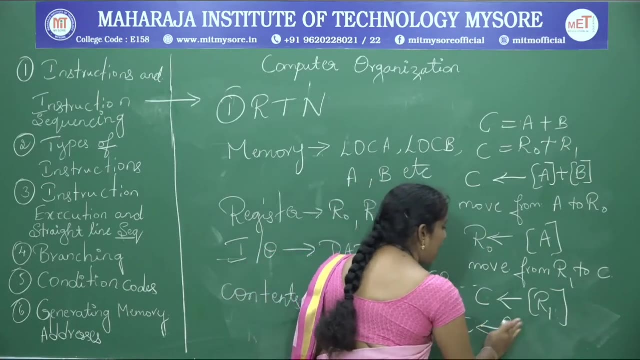 from R1 to C. right, okay. next you can say: C is equal to R0 plus R1, so here also C, content of R0 plus content of B. Okay, Okay, Got it. So here in the register transfer notation we are using capital letters to represent the 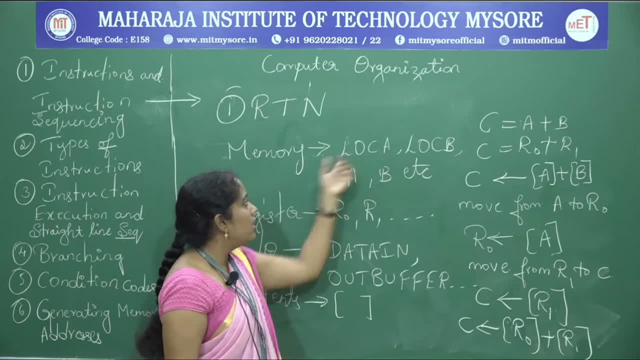 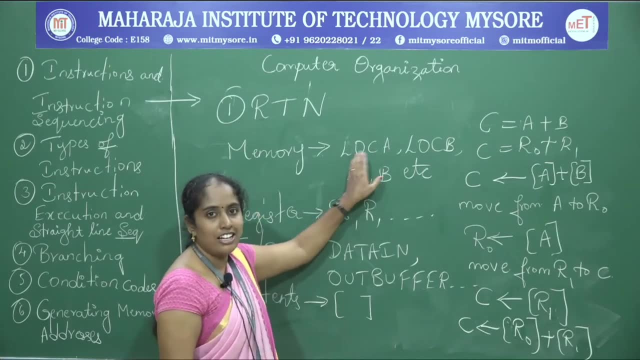 memory it can be memory name can be anything. so here I am taking simple examples for that location A, location B, A, B, etc. So for registers we are using R0, R1 and Rn right. so for input output operations, data. 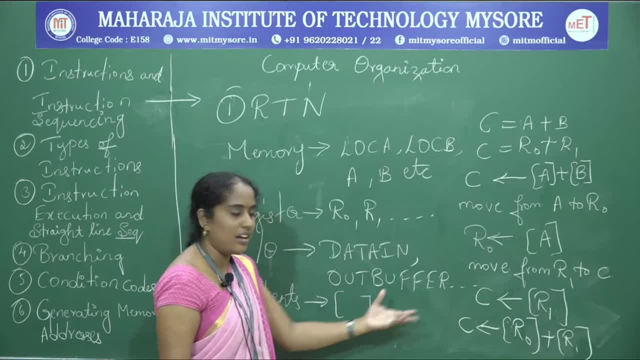 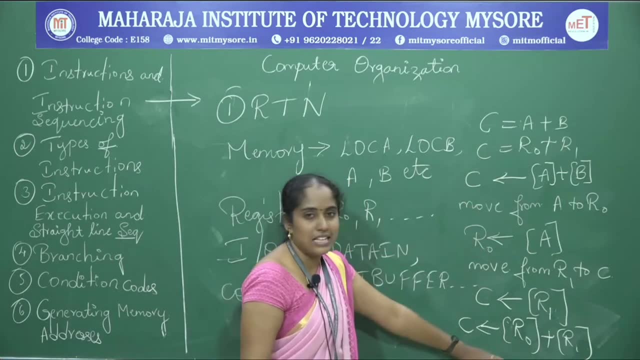 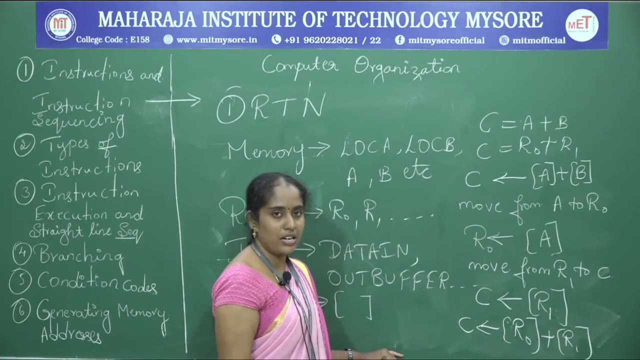 in data, out out buffer, in buffer, and so on. So the content will be represented by using the square brackets and this is the. this is the examples for that. Okay, So the second notation: yes, the register transfer notation. it is easy to understand. 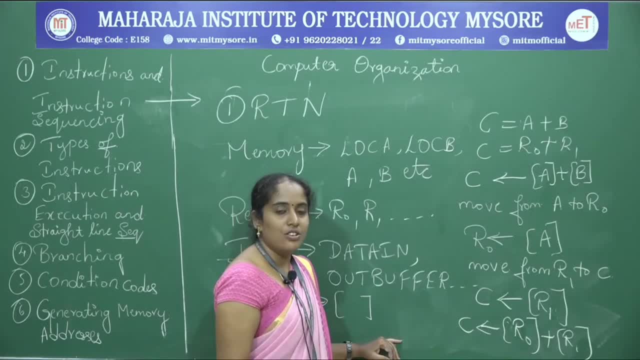 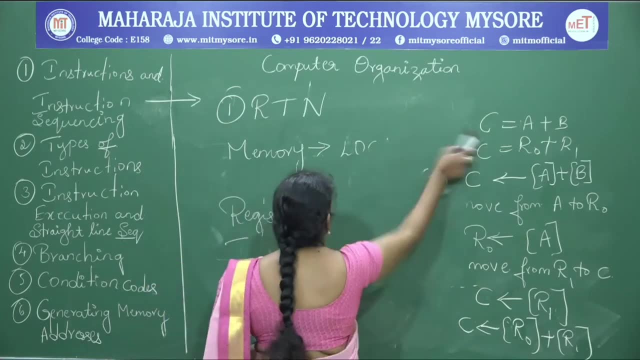 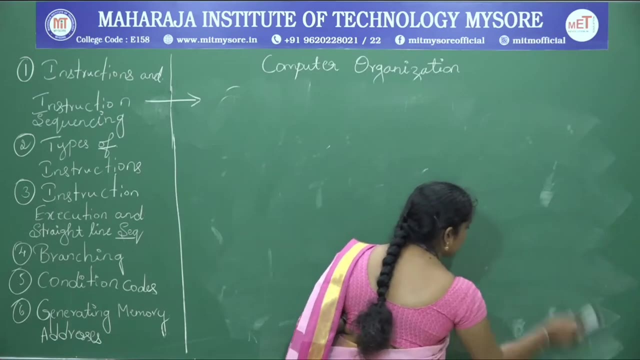 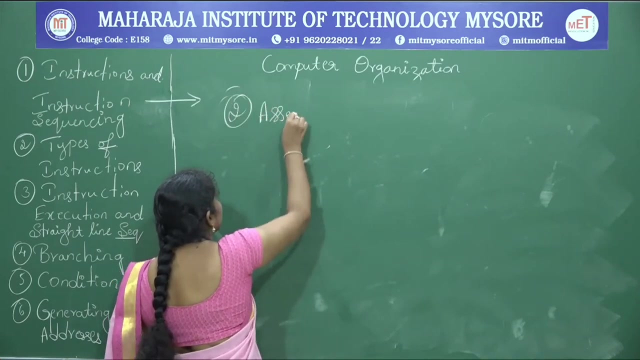 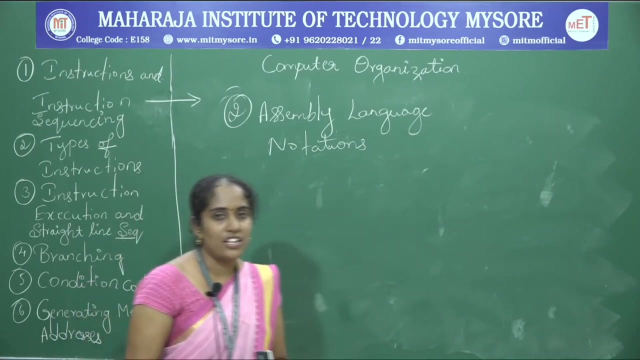 but we cannot write like this in the computer, So for that we are using assembly language notation. So next is the assembly language notation. Yes, so in the assembly language notation, first we use the, always we use the operation, and followed with the operands. 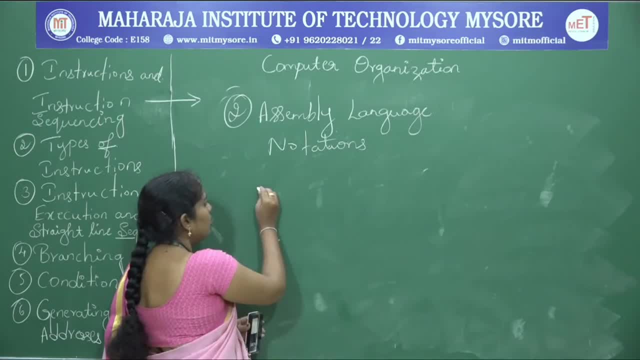 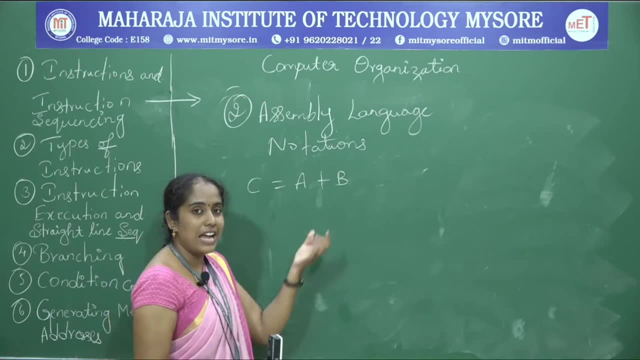 Okay, Say, for example, you want C is equal to A plus B, right Here how to write this. So for this addition, we are using add. add is the instruction, it is the operation, and add content of A with the B right. 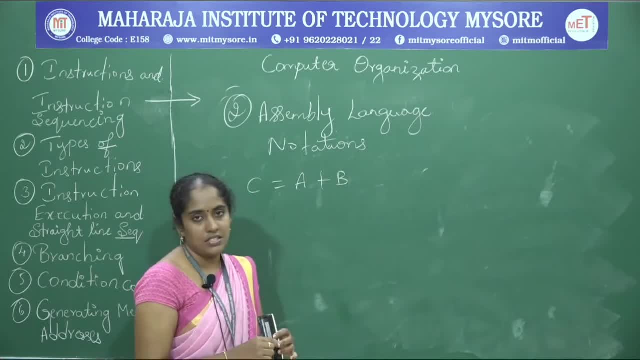 For that we use different operand names. Okay, Say, for example, this can be written as first: first you need to move this, A content content of A, to the any register that will be present in the processor. Here I am taking R1 register, or you can take R0,, you can take R2,, no problem. 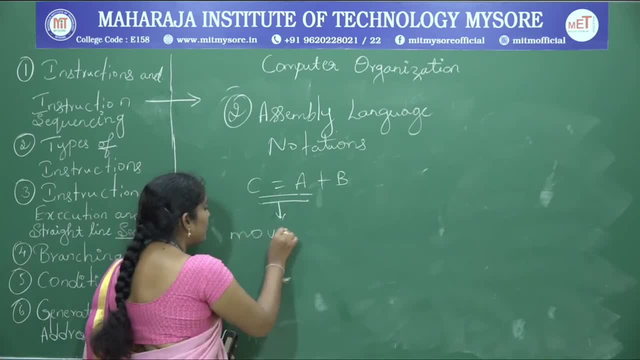 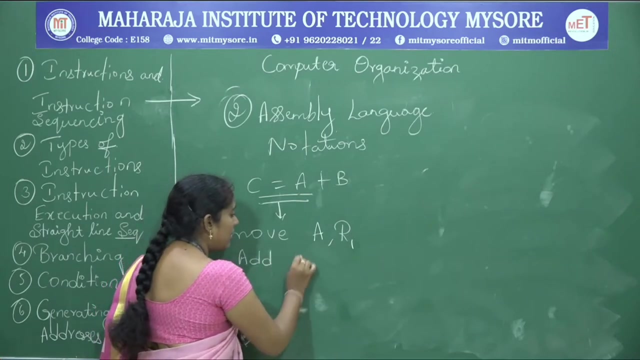 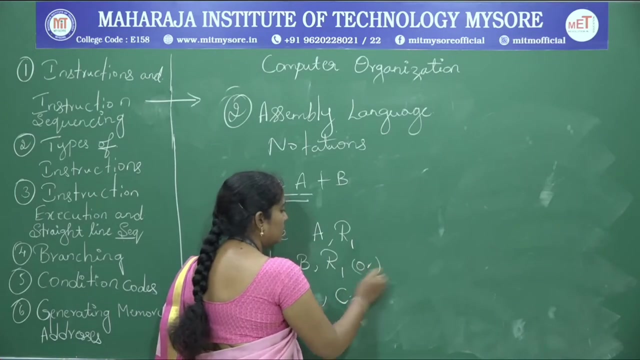 Okay, How Move? move so content of A to R0 or R1. Yes, Okay, Next add: add B comma R1.. And again, move, move R1, comma C. This is the instruction set. So, or else you can also write, yes, you can also write: move, move B comma R1. 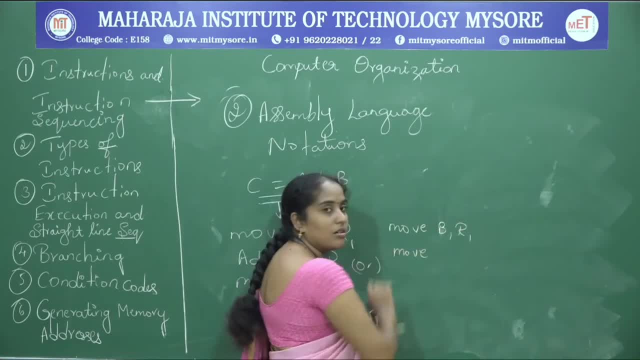 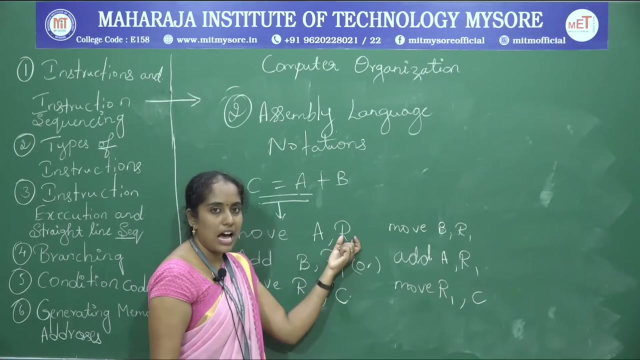 Yes, next is okay. sorry, next is add: add R1, sorry, A comma R1. And move R1 comma C. Both are correct right Here. first you need to move the content of A and store it in R1 and add the content of. 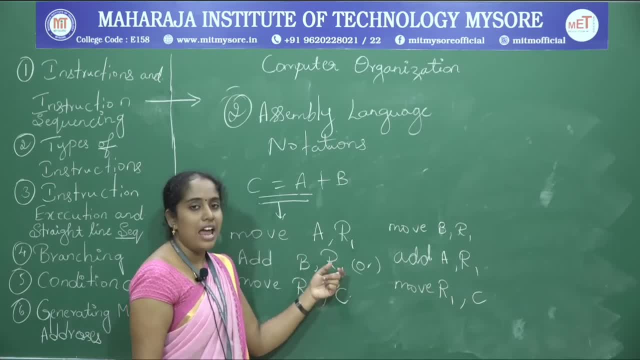 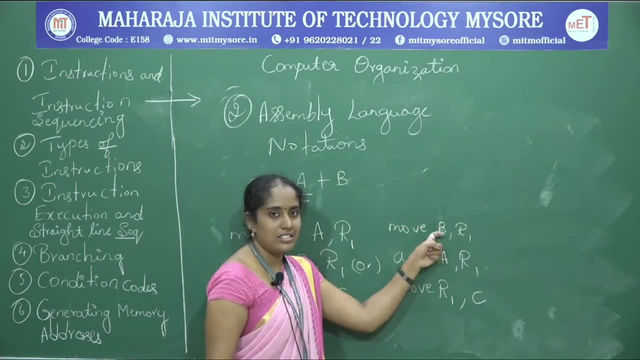 B with the content of R1 and store the result in R1 and move this R1 again back to the memory C right Here. yes, only this step is changed Here. move content of B to R1 and add content of A with the R1, R1 contain the value B. 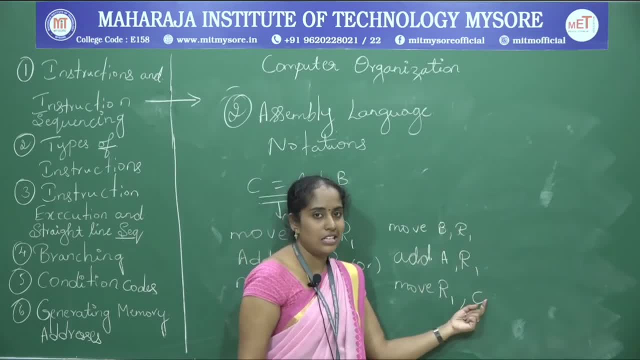 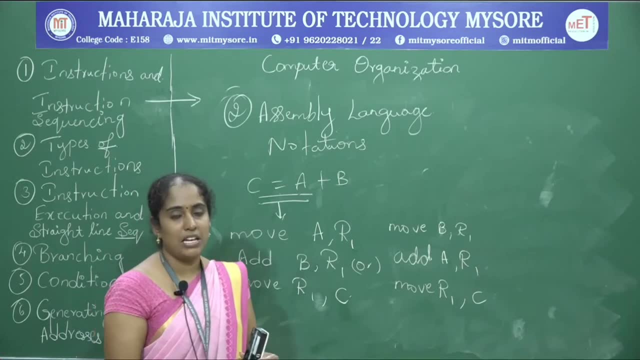 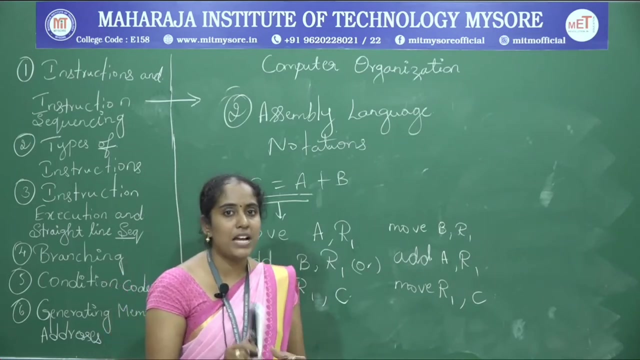 Then the result again will be stored in the C right. This is the assembly language notation. So here the main disadvantage of the assembly language notation is it is not portable, It is a. it is a depends on the processor right. It depends on the processor. 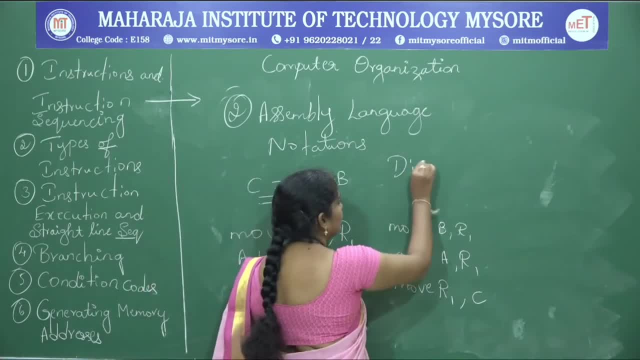 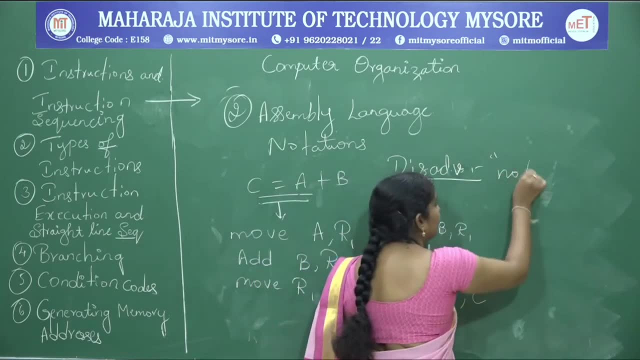 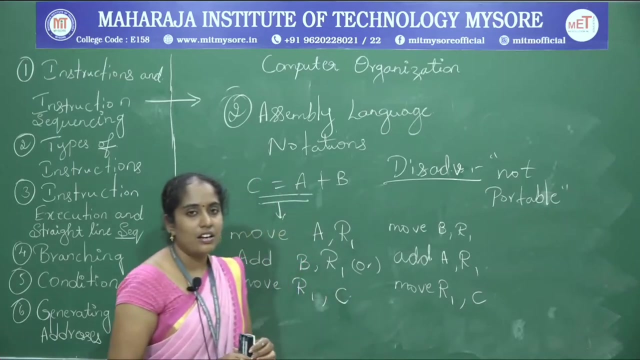 So the main disadvantage is Okay. This advantage is it is not portable. So for that reason, for that reason, we are not using the assembly language, right? So instead of that, we are using the high level language to write the program Here. high level language, it is a machine independent. 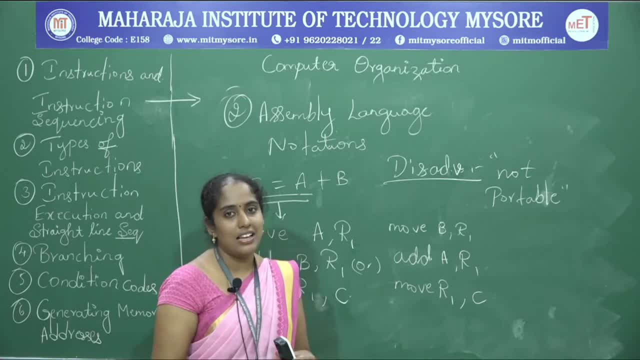 So for that reason we are. we are writing any program in a high level language, not in the assembly level language. Assembly level language. it is not portable. It depends on the processor. okay, So this is all about the instruction and instruction sequencing. 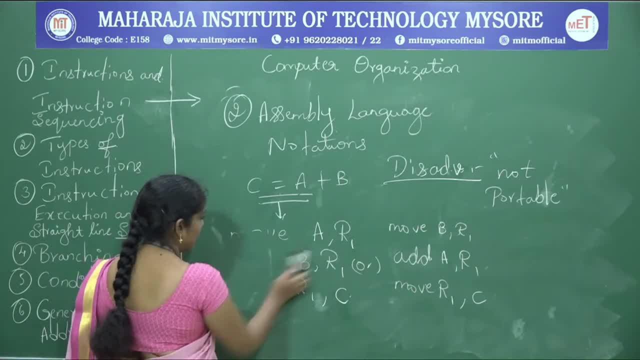 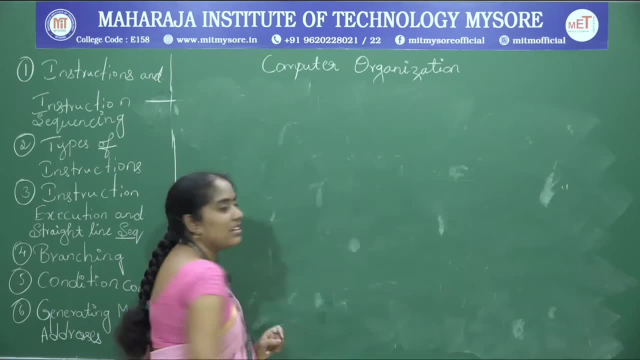 So the next topic is types of instructions. Next it is a types of instructions. So in this types of instructions, here the it depends on the, this type, it depends on the number of operands, How many number of operands we are using or we are showing in the instructions. 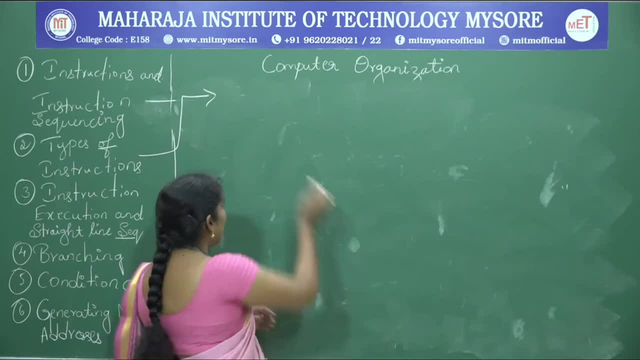 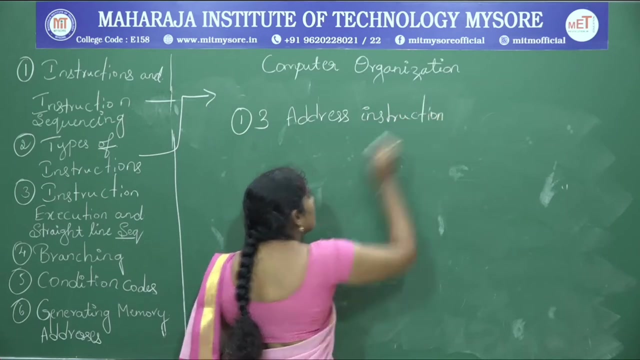 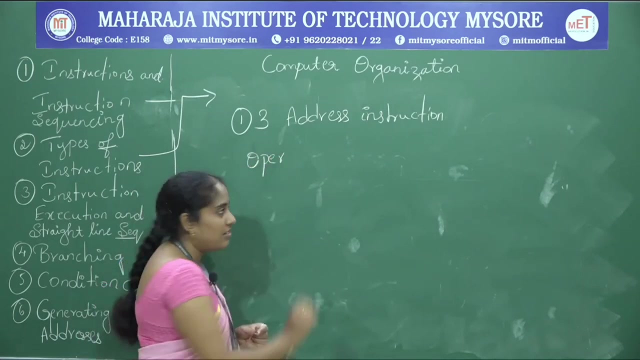 Okay, So in that first one is a three address instructions. What is that? Three address instructions? Okay, So in the three address instructions here the format for the syntax is operation and the source one comma. source, two comma. Okay, So this is what we are not using for the syntax. 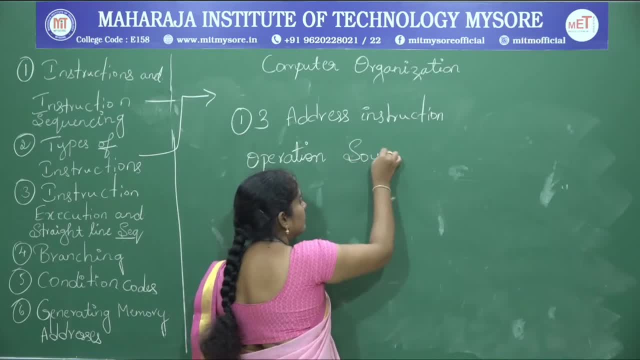 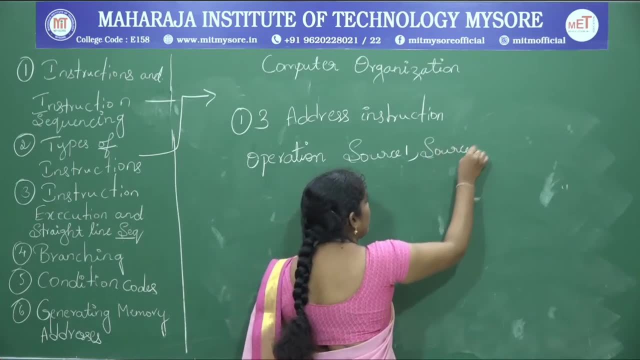 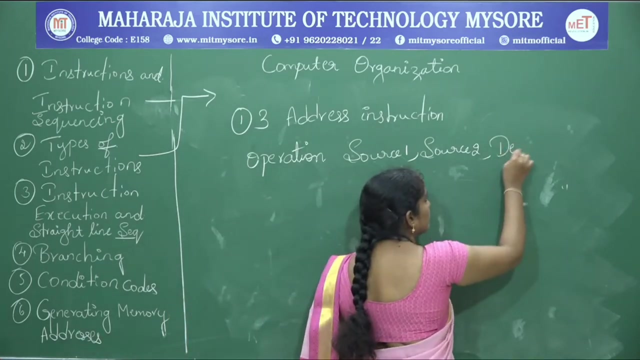 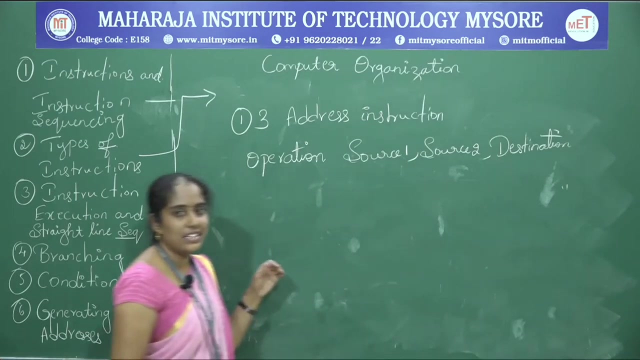 This is exactly what we are using for the syntax. What will we be using for the syntax? This is exactly what we are using for the syntax. All right, So this is it, comma, and the last one is destination. this is the syntax for three address. 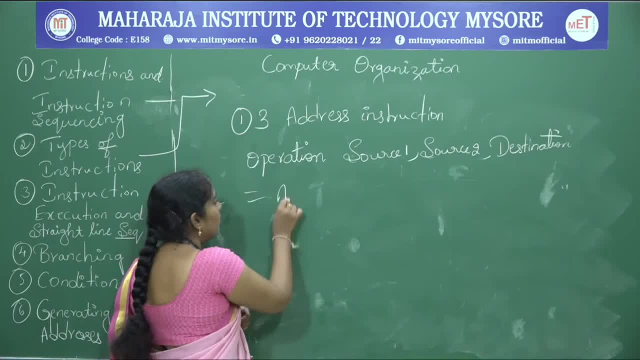 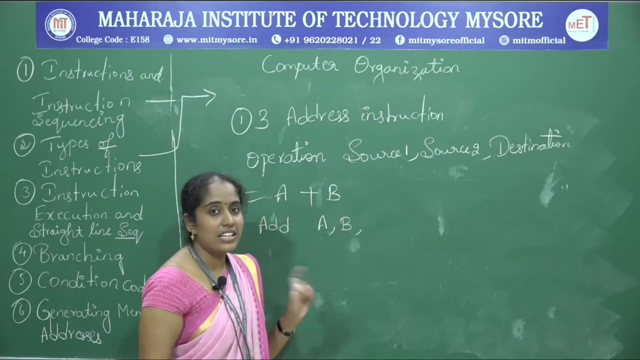 instructions. example for this is: C is equal to a plus B right. so here operation is addition. so add here source 1 right. source 1 can be a right, a comma, source 2: it is B and the destination is C. so we cannot directly write like this: 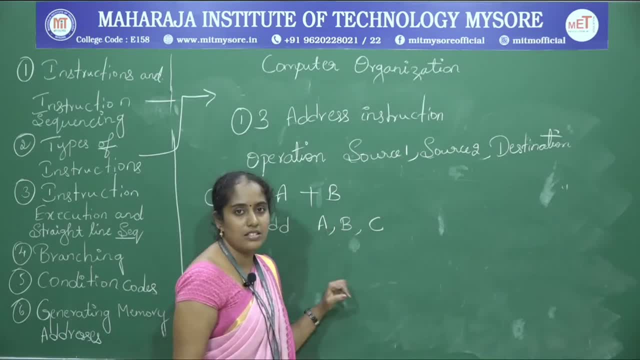 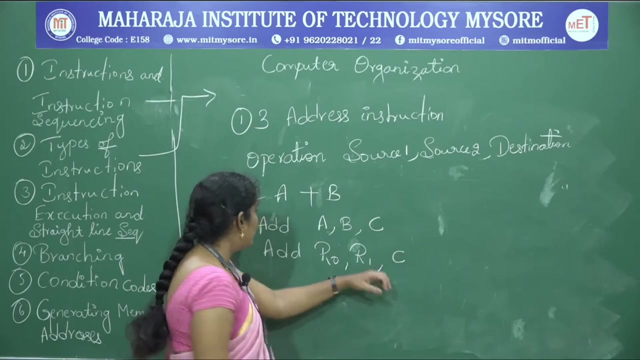 because you need to move this value into the register. so for that reason I can write like this also: add: add r0 comma, r1 comma C. right, so in this example? so r0 contain a value, r1 contain B value. add these two and store the result in C. ok, so next is the or else. 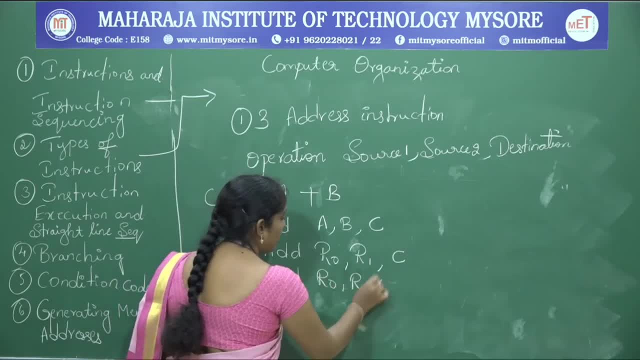 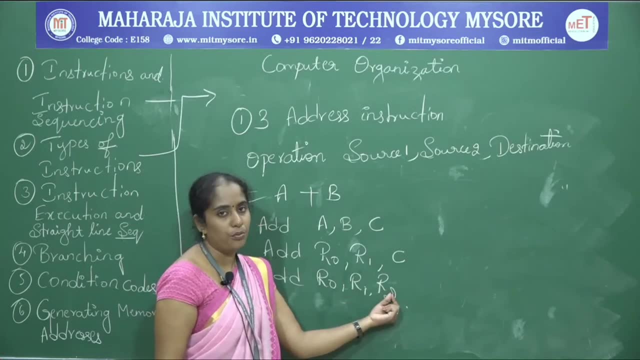 add r0 comma r1 comma, r2 here. also add r0, r1 value and store the result in r2. ok, so here we are not using the three address instructions. yes, it contains only one line right to addition of two numbers. it contains only one line, but. 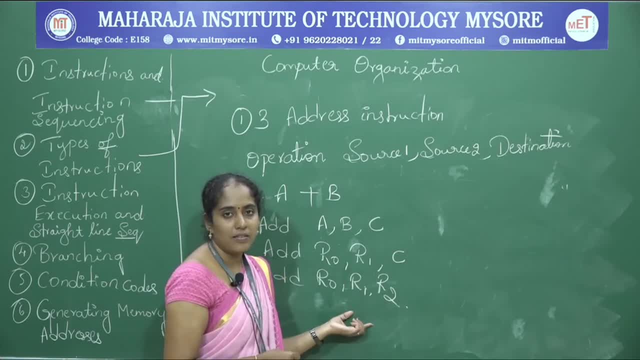 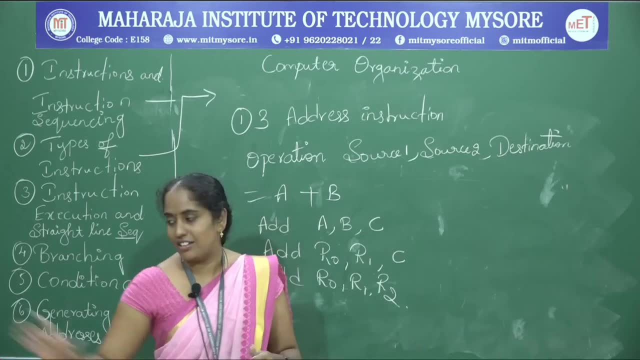 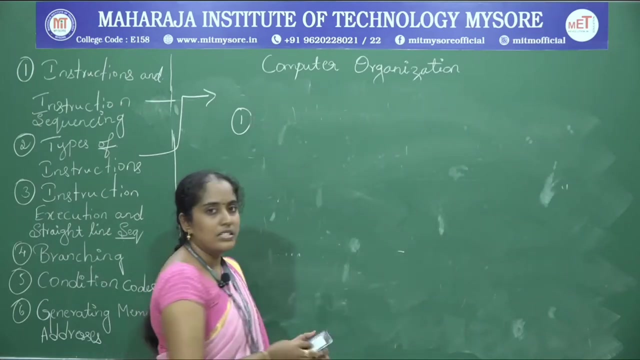 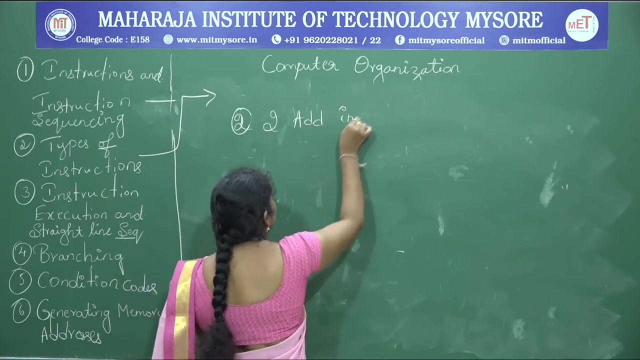 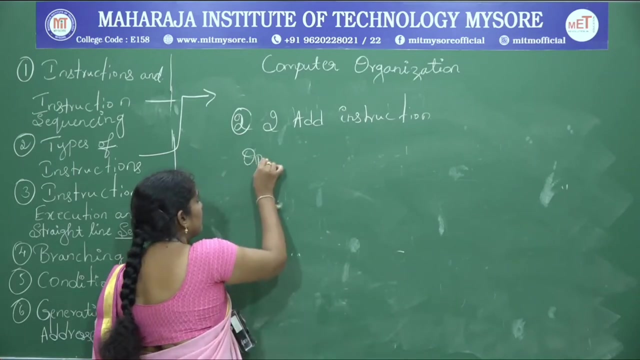 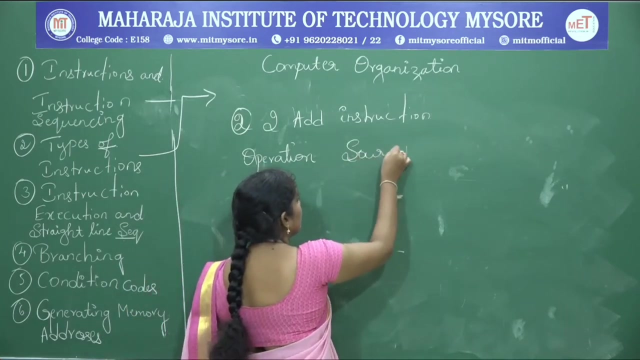 you cannot fit this into the one word in the main memory, so for that reason we go with the second one. second type: second one is a two address instruction, yes. second one is to address instruction. again, the format for this is operation. here it can be source or destination. 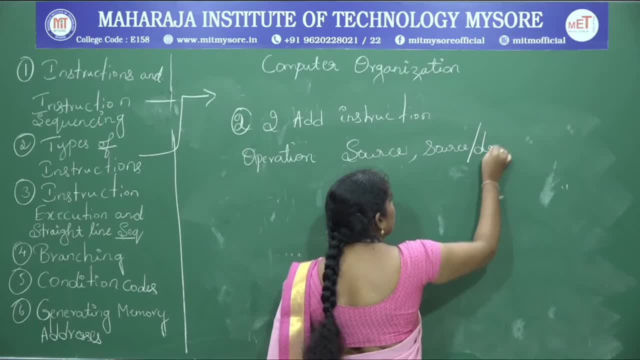 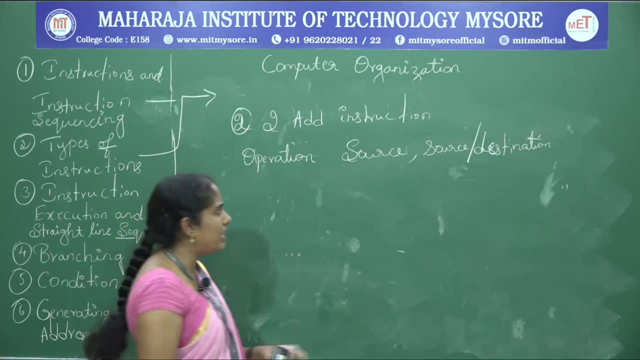 Ok, I'll tell you why. it is source or destination. Again, take this simple example: c is equal to a plus b, So in the one instruction you cannot perform the addition of two numbers, So for that we need several instructions. 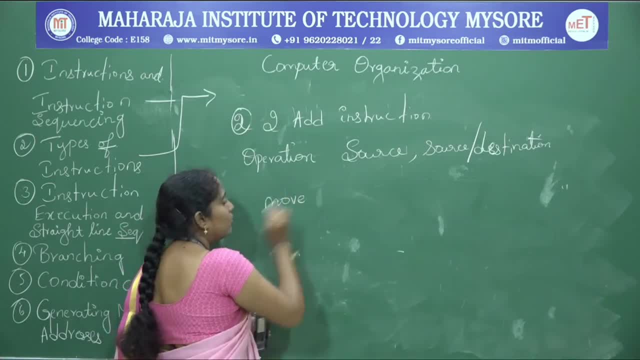 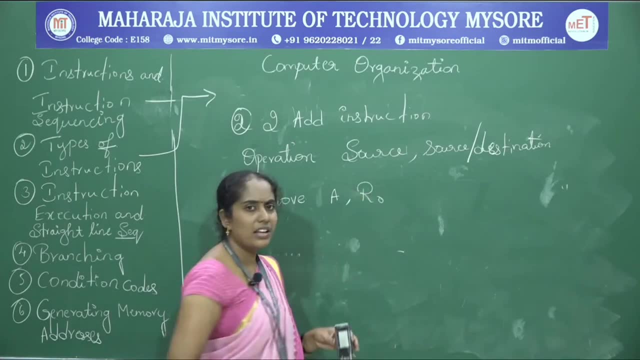 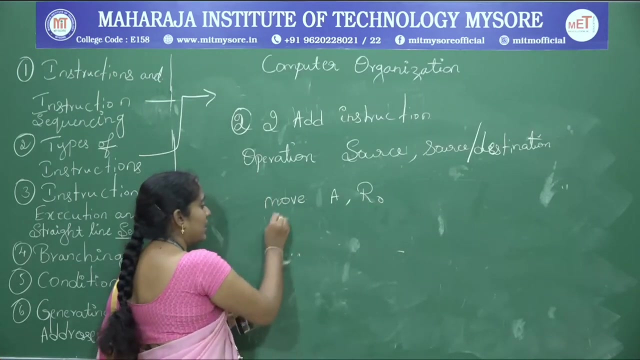 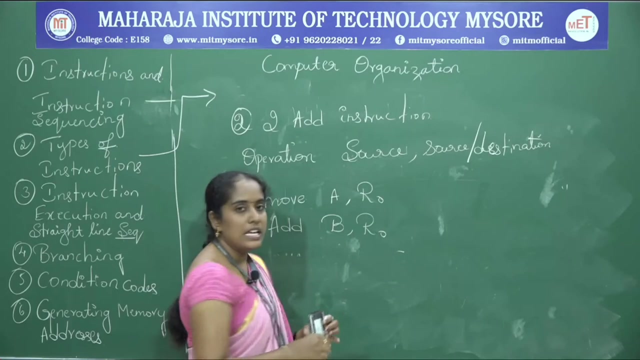 For example, move first content of a with the r0. Right, So here a is the source and r0 is the destination. Right. Next is the add addition: Add b comma, r0.. Here you need to add, you need to take the two volumes, one from the b and another. 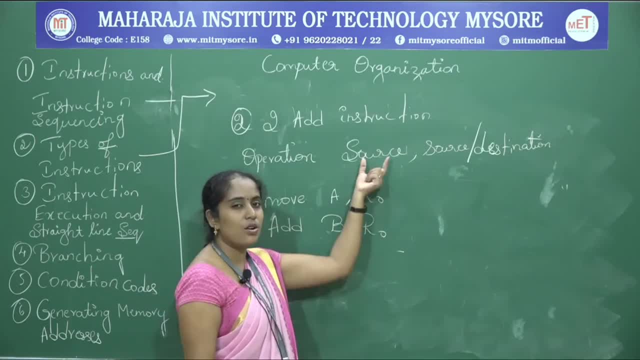 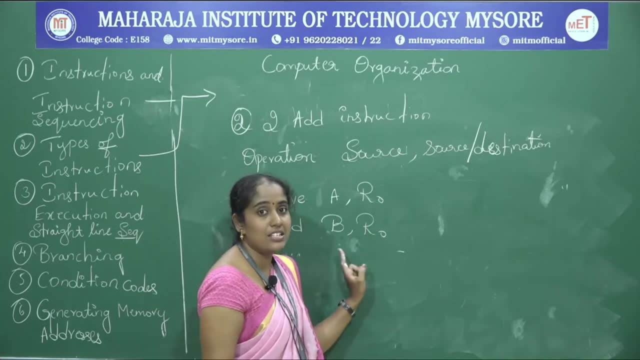 one from the r0.. So here b it acts like a source, Yes, but r0 it is first it is source and add these two numbers and store the result in r0.. So here it can be act like source as well as the destination. Okay, 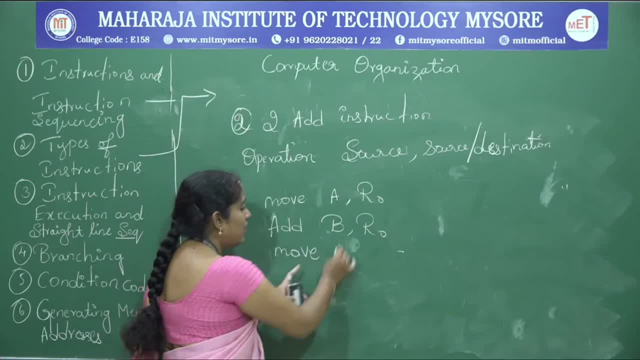 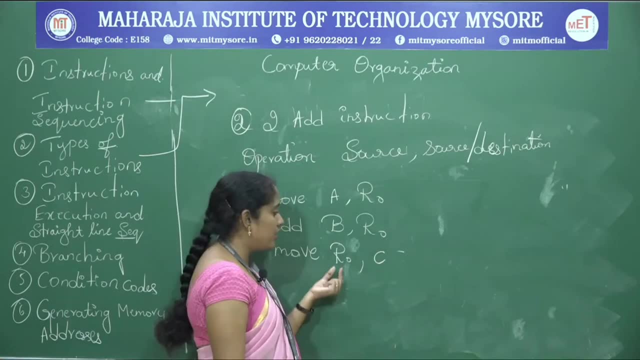 So next is move r0 comma c. Here r0 is a source and c is the destination. Here you need to store the r0 value into the destination, Right. So here you need to store the r0 value into the destination, Right. So here you need to store the r0 value. 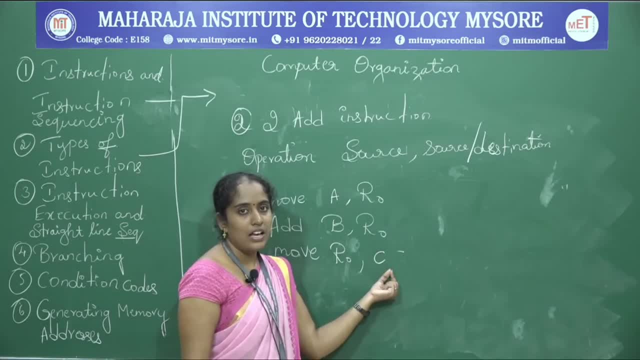 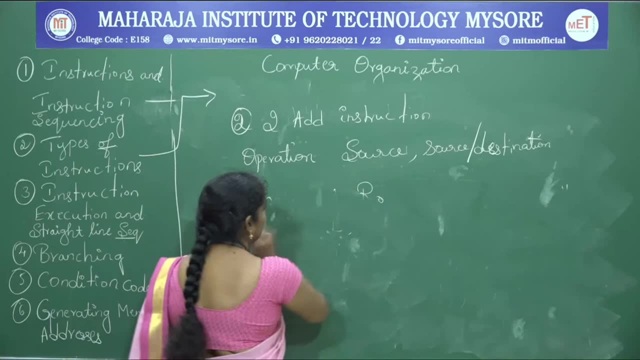 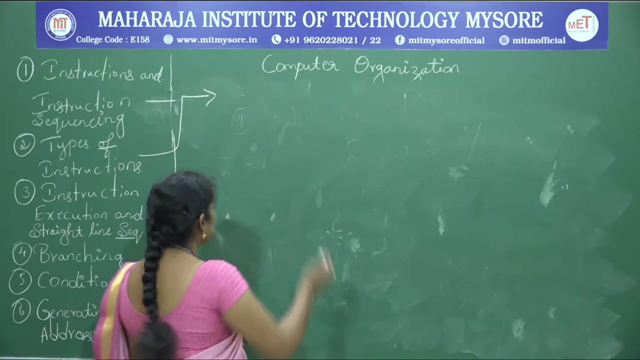 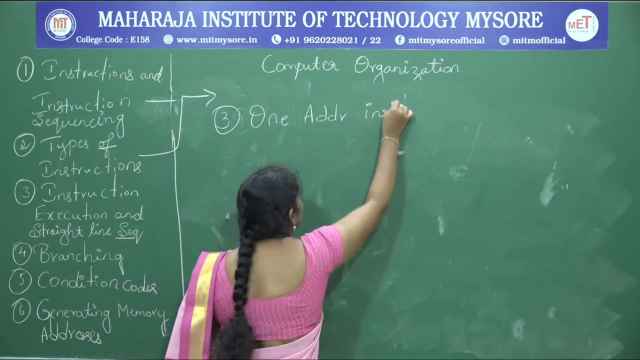 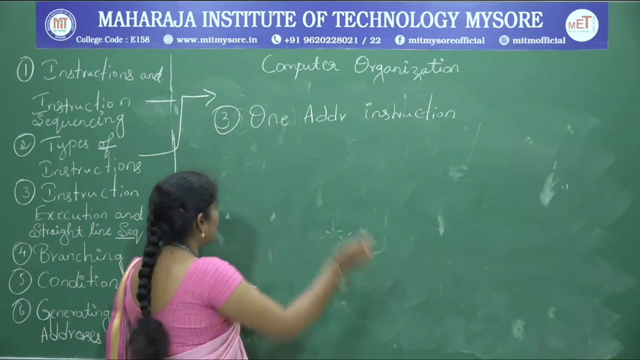 to C. The result will be stored in C. Okay, This is the two address instruction. So the next type is one address instruction. So third type is one address instruction. Okay, Here in the one address instruction. so first is the operation and it contains it may be. 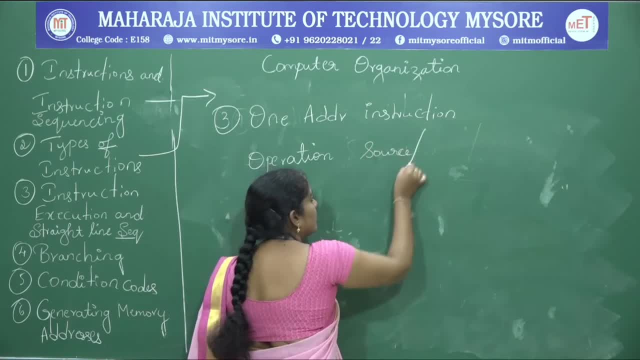 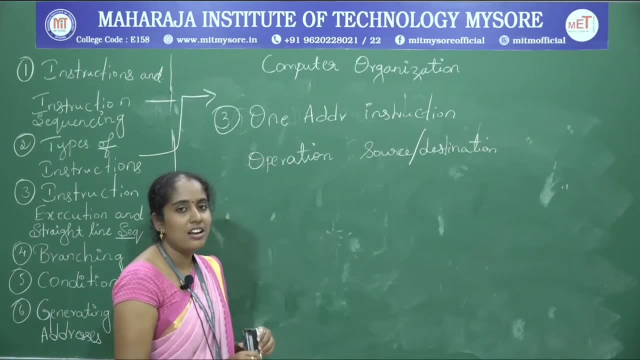 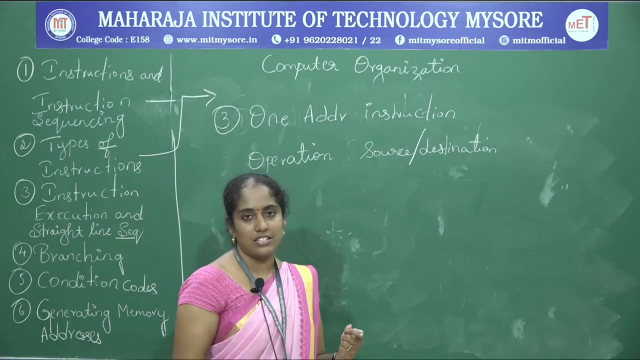 it is a source or destination. Okay, Source or destination Here in the one address instruction format, so the other one is. so one is source, another one is destination. Right, So other one it is we are taking explicitly, So your computer will take the other one. 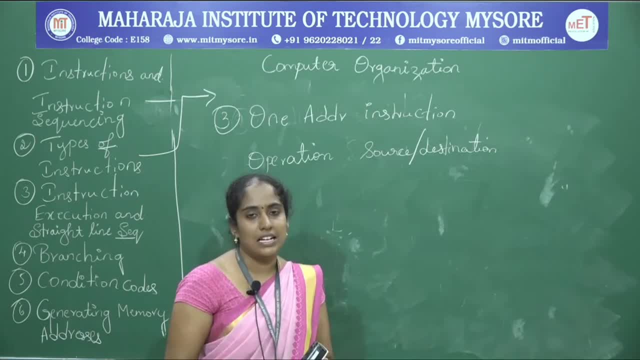 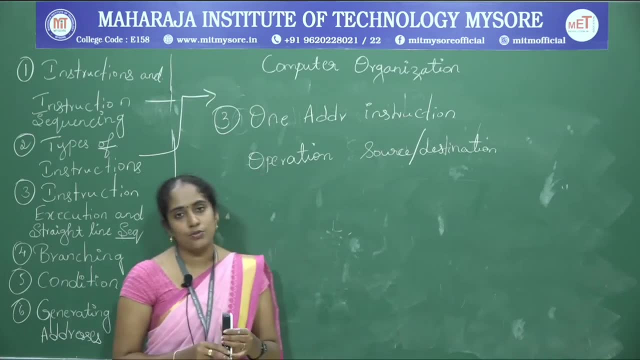 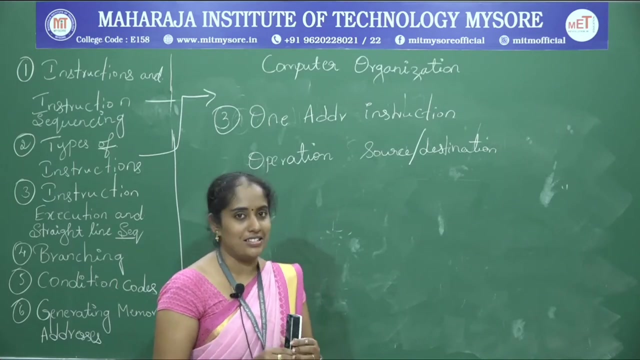 So it can be source or it can be destination. So implicitly Here it will take the accumulator register, So accumulator. it is mainly used for automatic and logic operations, So it is a special register present inside the processor, So it is that name, It is accumulator. 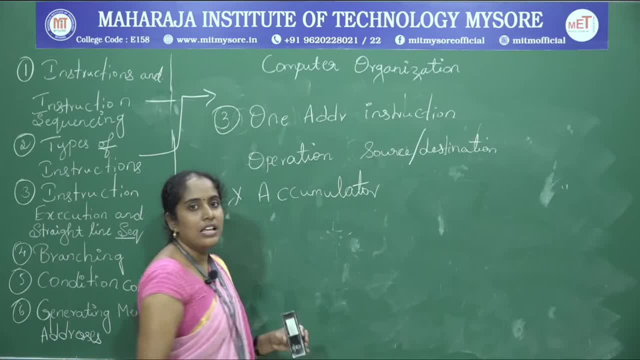 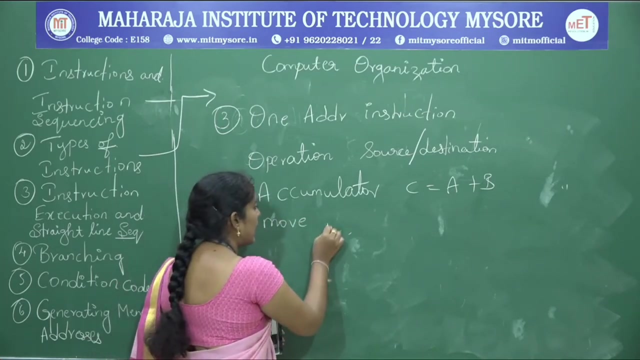 Okay, Take an example: addition of two numbers: C is equal to A plus B. So how to write this? in one instruction? Say for example: move, move A. So here you move the content of A to the accumulator register. Here it will move the content of A to the accumulator register. 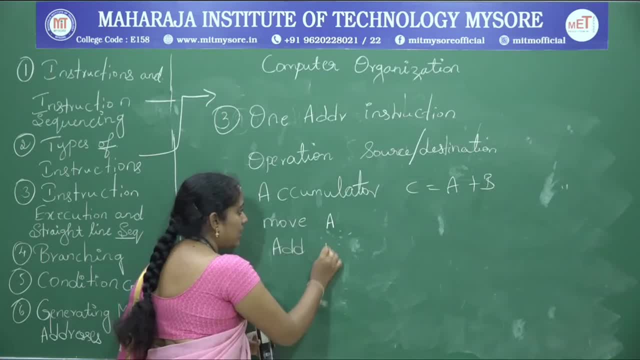 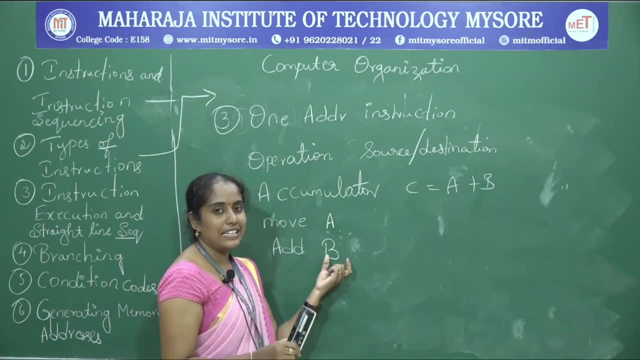 and the second one is Add B. Here it will add the instruction. So add is a instruction. It will add the content of A, B with the accumulator register and the store the result in accumulator register. Okay, So the next is move C. Here it will store the value result from accumulator register. 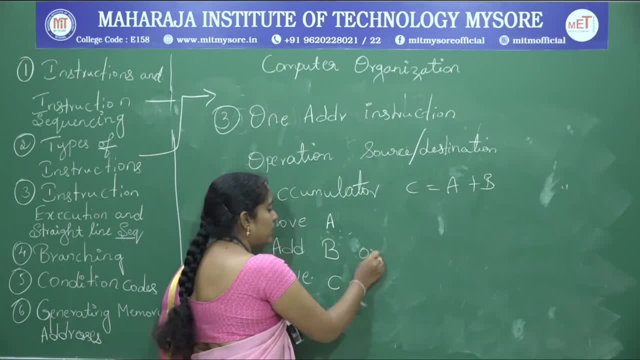 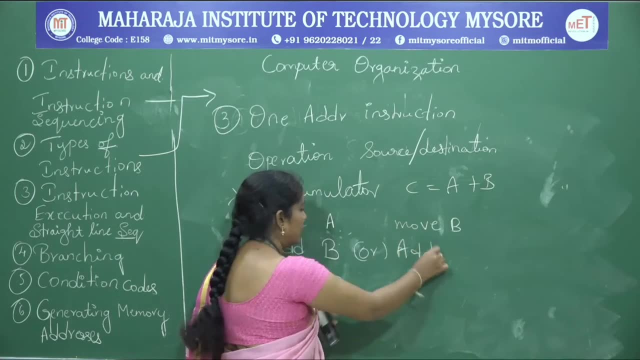 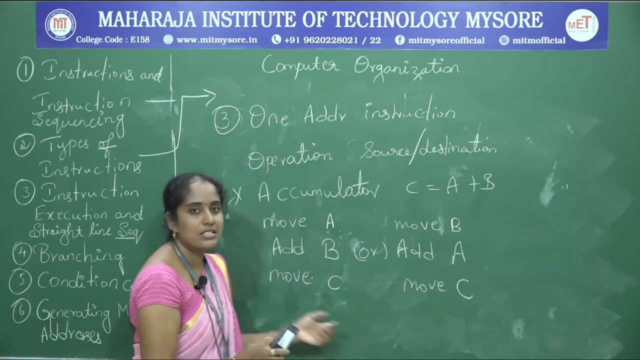 to C. Okay So. or else, And it can also be write like this: Move B and add, Add A and move C, Both are same, Okay So. first you need to take the A content and it will move to accumulator and here add. 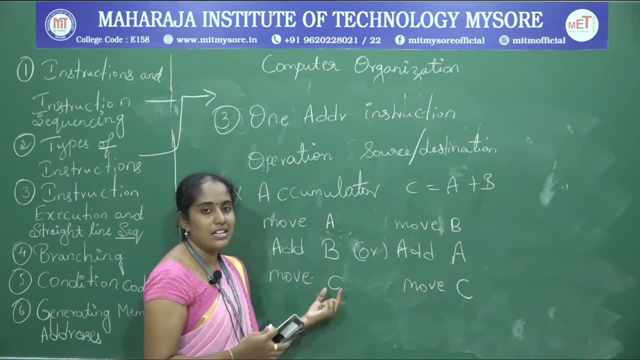 content of B with the accumulator And next the store, the result in C from accumulator, accumulator to C, right From accumulator to C. Similar way, this is also same. First we take the, we move the content of B to accumulator, add A value with the accumulator and store. 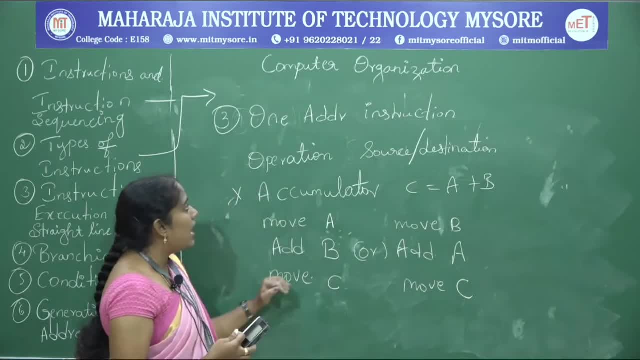 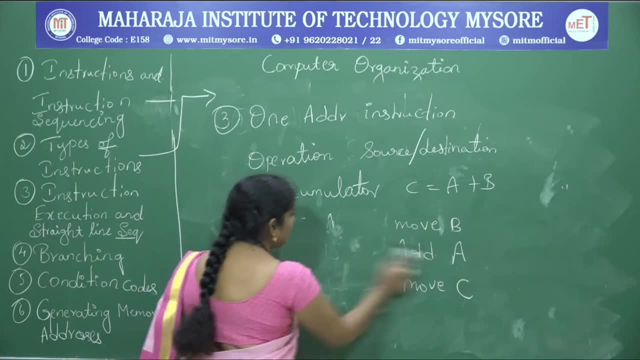 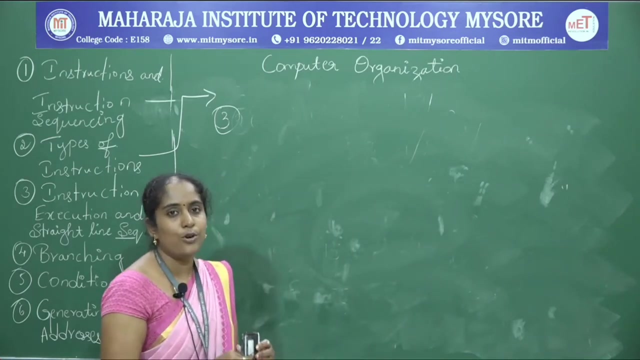 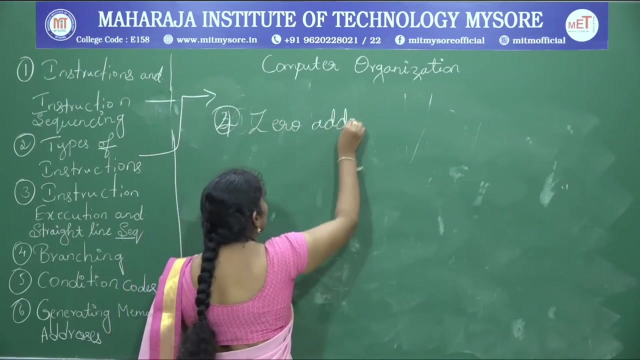 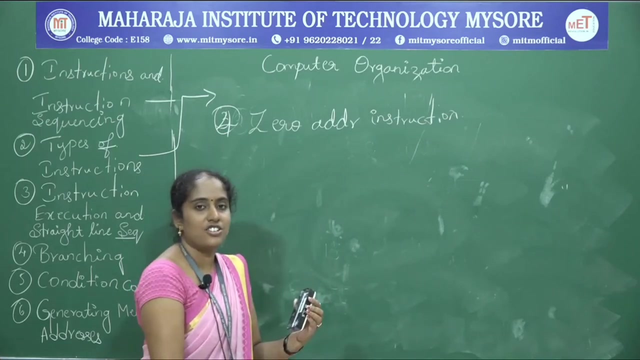 the result in C. ok, This is all about the one address instruction And the last one, last type, is zero address instruction. The last one is zero address instructions. ok, So in the zero address instructions. so both source and destination it has defined implicitly. 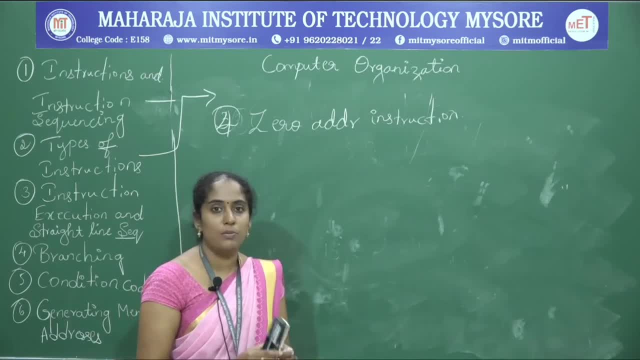 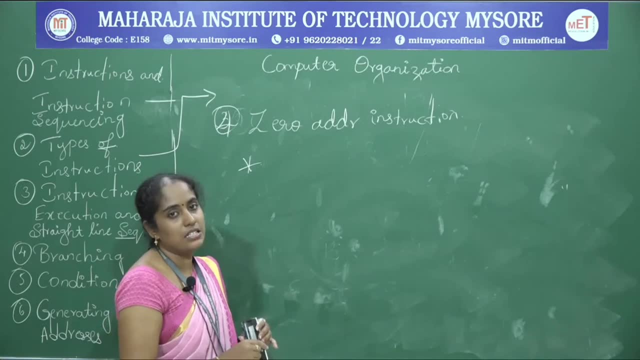 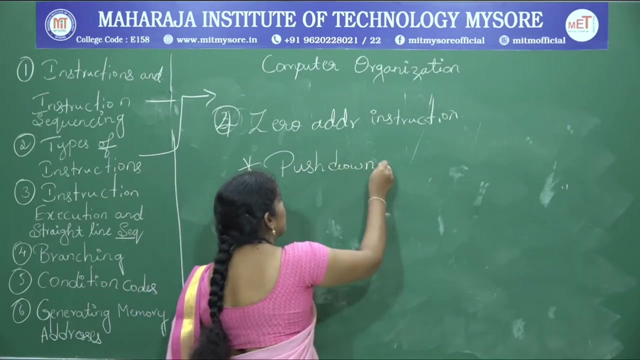 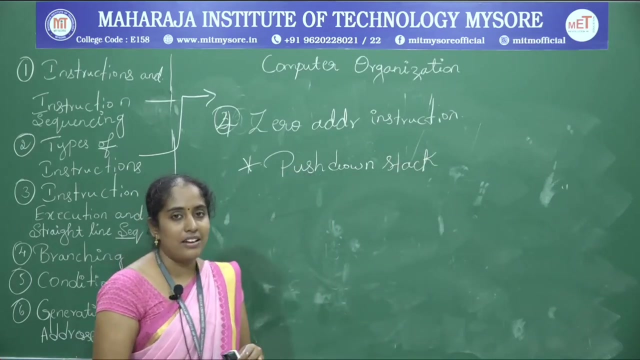 right. So here the operands, operands, value- will be stored in the push down stack. Here the content or the operands will be stored in the stack With stack, push down stack. So in the assembly language we are using two address instructions. It is very familiar. 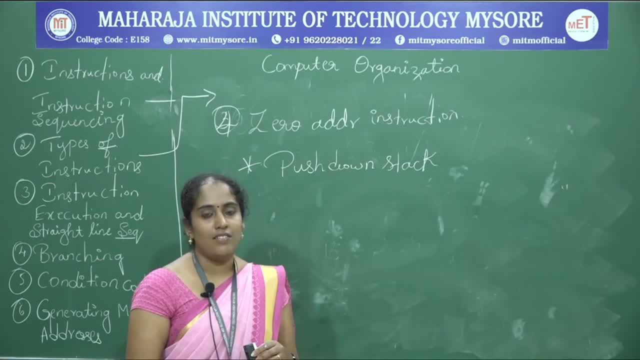 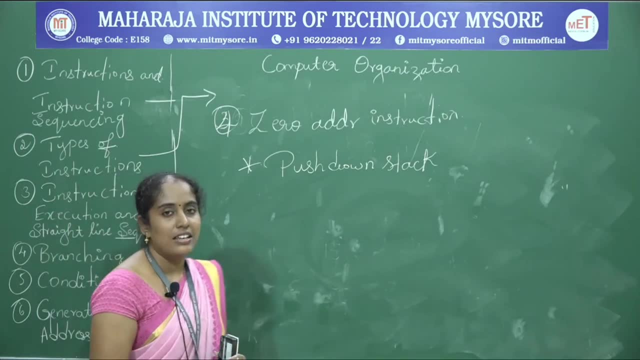 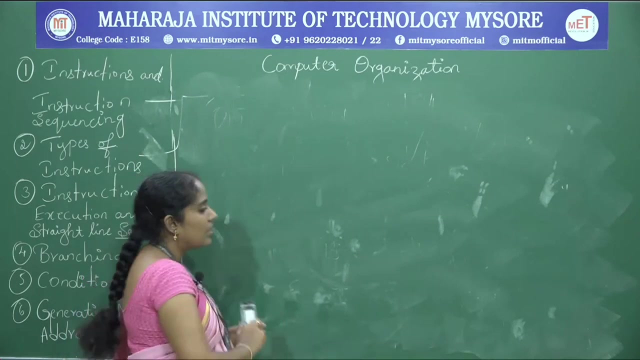 and it is easy. ok, So we are always using the two address: instruction. ok, This is all about the types of instruction. Next, we will move to the next topic, that is, instruction, execution and straight-line sequencing. Ok, Instruction, execution and straight-line sequencing. What is this? 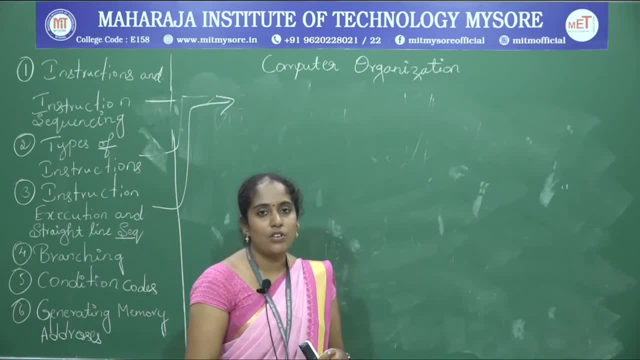 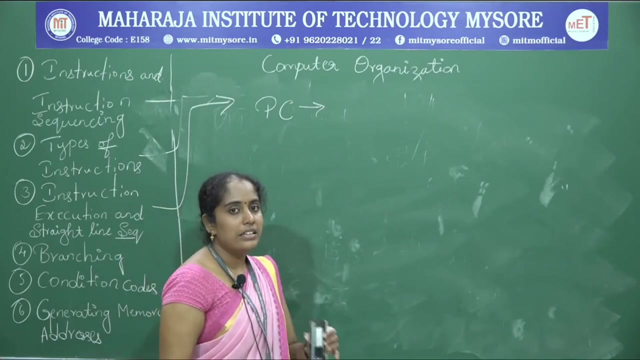 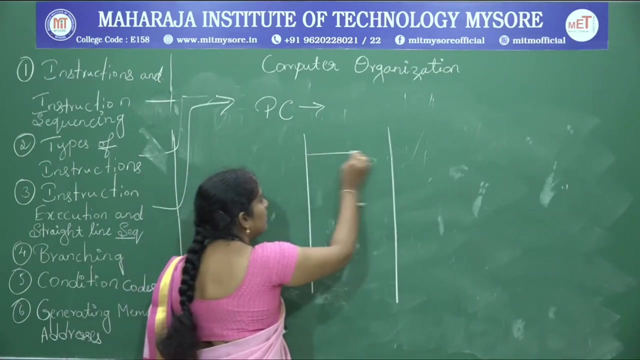 So, as we know that always the program counter, it will contain the next instruction, it will contain the address of the next instruction to be executed, right. So PC will contain the address program counter, right. Take an example: this is your memory, this is your memory here. this is the word right. 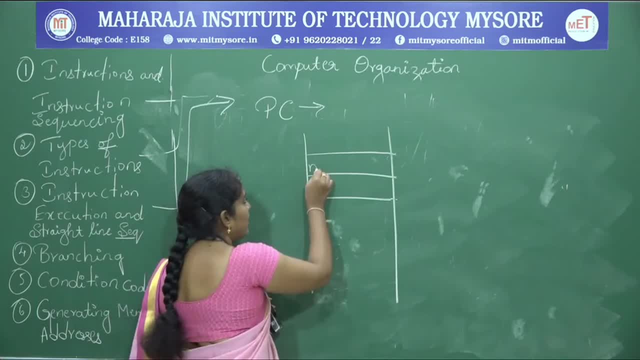 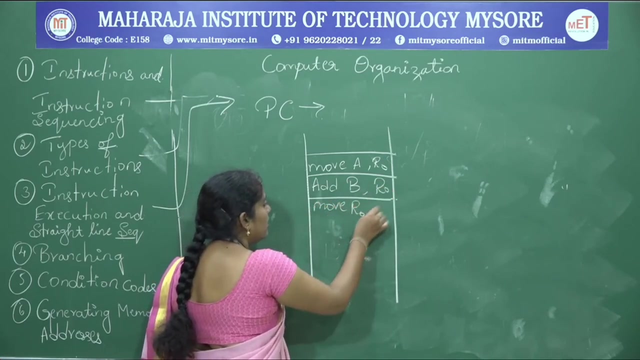 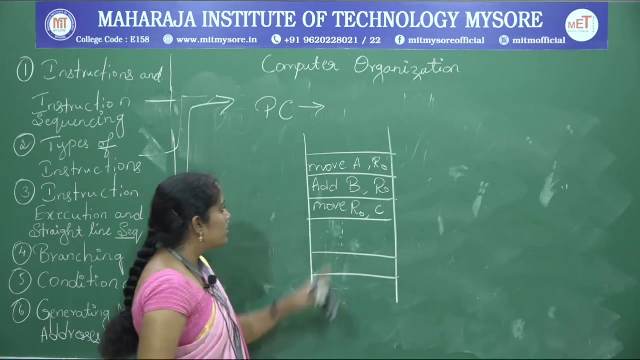 Take an example of addition of two numbers. so first move a comma r0 and add b comma r0 and move r0 comma c right, And so the a value will be stored here like that, And so the b value will be stored here like that. 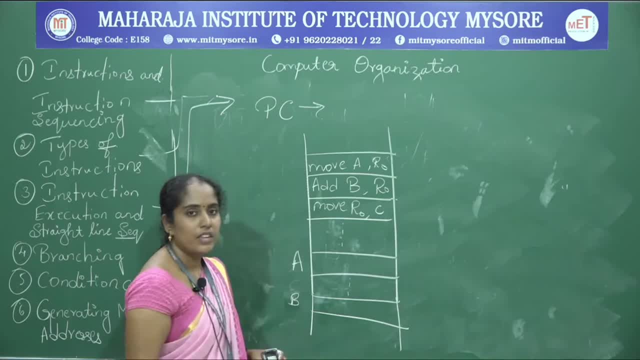 And the b value will be stored here and the result may be stored here: c- okay, This is the content of a. this location, this word, will contain the content of a and this location will contain the content of b, and this is the final result. c is equal to a plus b, right? 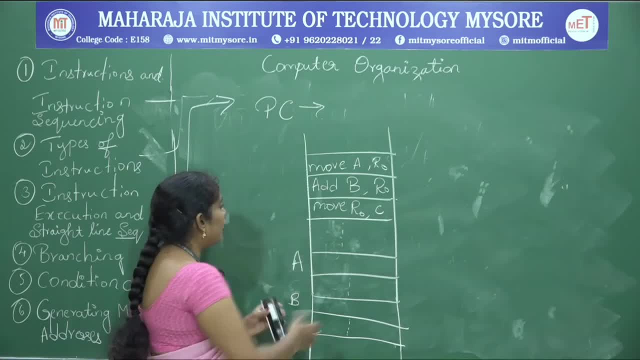 C result will be stored in this place, right? Say, for example, the address of this is a- I. okay, The address of the first instruction may be i and the next instruction if it is a 32-bit word length. in that case, what is the next address? 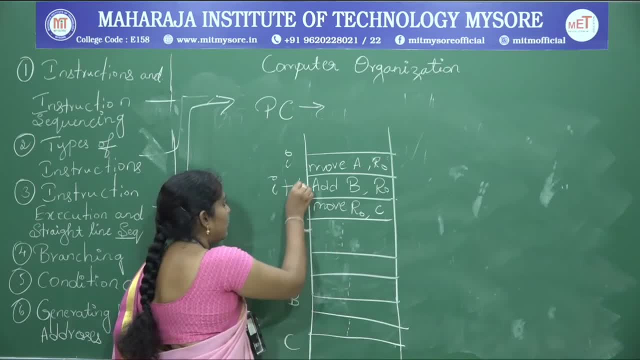 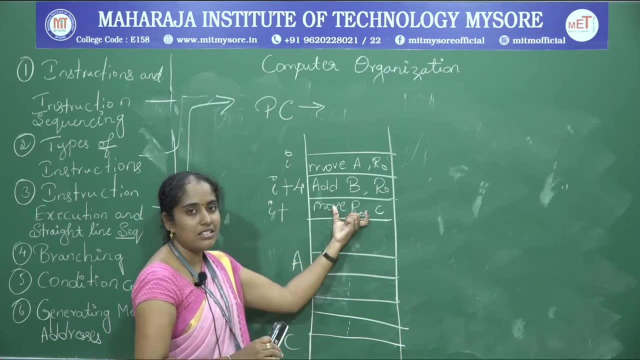 It is i plus 4,. okay, I plus 4.. So it is a next instruction address. next word, this word address: it is i plus. so add plus 4 here. right, It is 8, and so on. 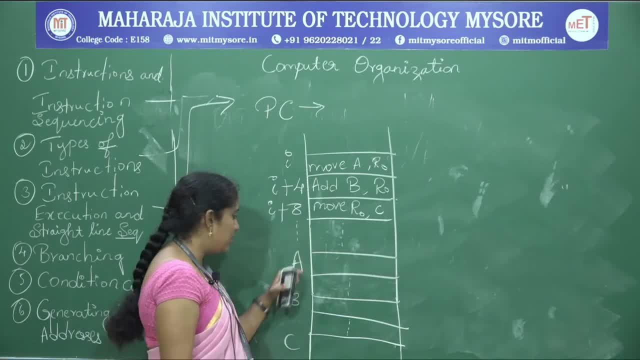 Right, So this address may be this: a value may be stored in another location. this is in another location and c for result, it is in the another location, right? So here this is the instruction to compute the addition of two numbers, and this is a and b. this value, right. 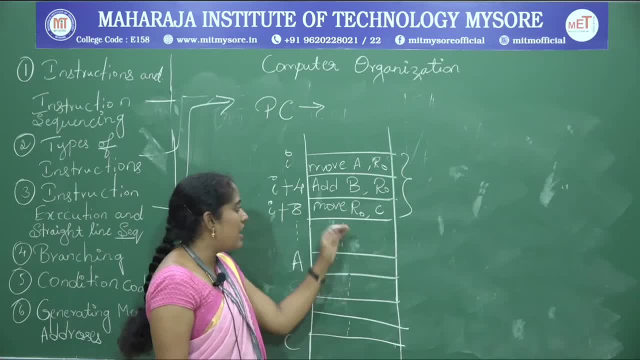 a and b value will be stored in this location and this location Right, And after the computation, after the addition, After the addition of two numbers, the result will be stored in this location right, Always. initially, the PC will contain the value i address of i. 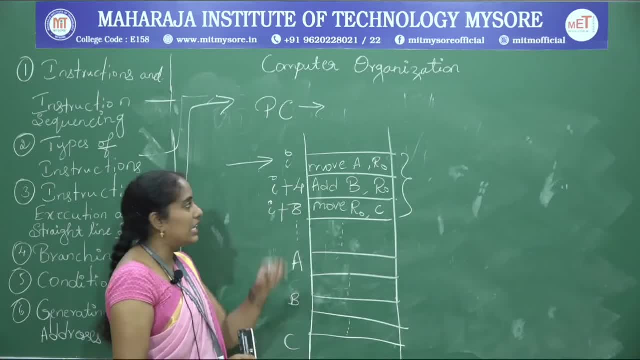 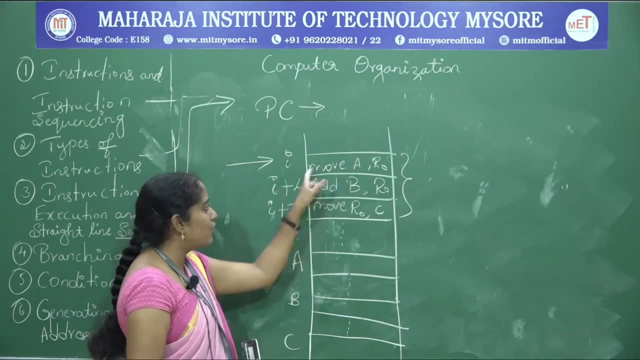 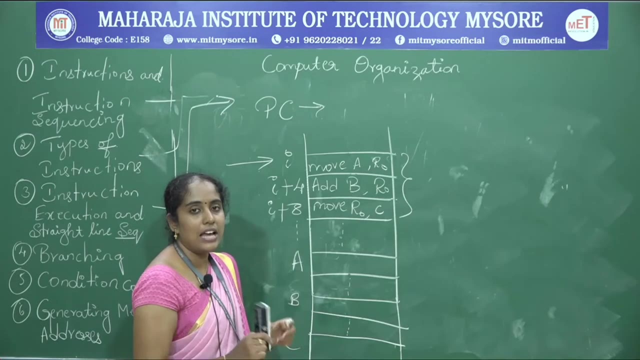 So always the program execution is begins in this location, from this location, right i. So PC will contain initially i and we move this whole instruction into the whole instruction into the processor. So in that m, a, r and md are like right. 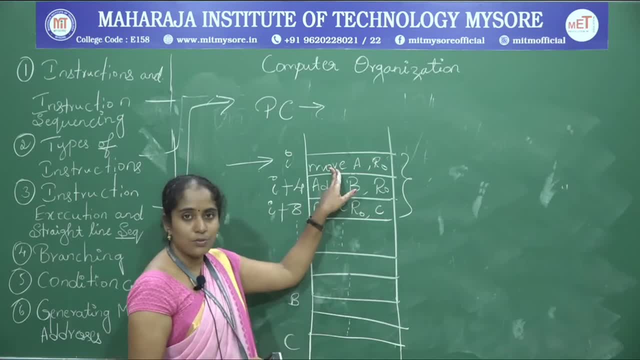 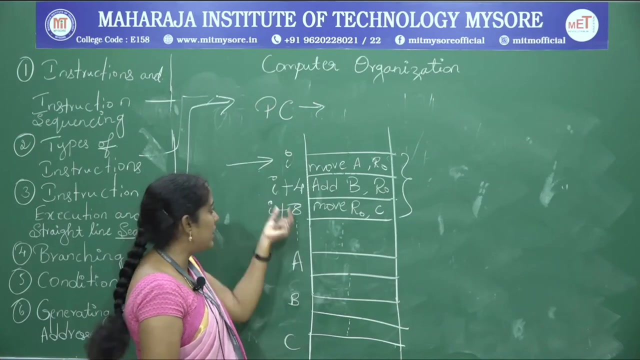 So md are memory data address And in md they have a sub接下來 of md and the upper Titans, Md are the残 Walker for Each record set. Now md and a higher S. So md and and they have a've world data. they have, they have a new engine. Northeast tower. So look in this corner, pointudge Now inside control center. It will contain: first it is move and move. yes, yes, it is the instruction. you will see, you will identify this is a instruction and it will send this move instruction to the IR instruction register. SO once it moves IR move into the IR register, your program counter value will be incremented. 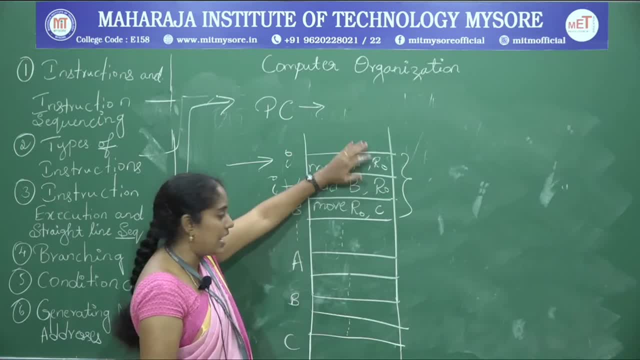 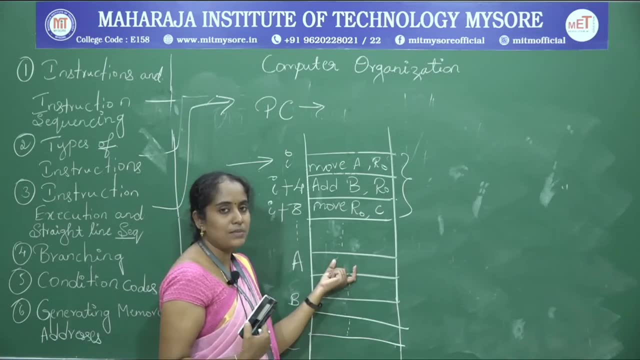 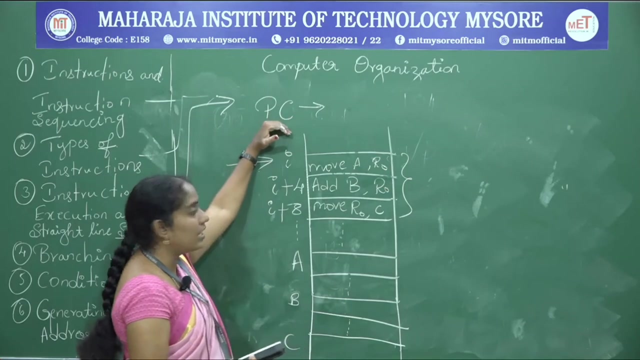 take the A value, it will search the content of A in this memory location and find out the location and it will take the data from the memory in this memory and store it into the register R0, right, So after that again it will check. it will check. So PC contain. 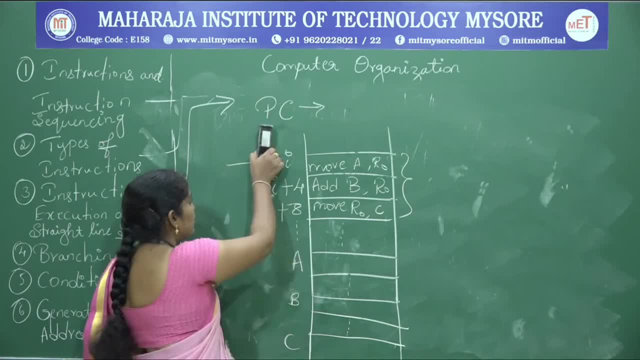 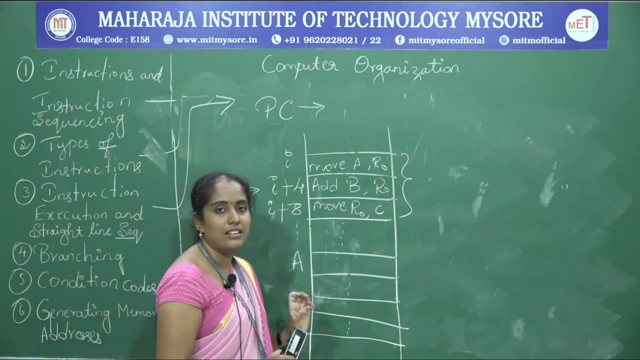 the next instructions: right. Next instruction address. so that is I plus 4, right. So here it will execute sequentially. that is why it is called as. that is why it is called as straight line sequencing. that is why it is called as straight line sequencing. executes. 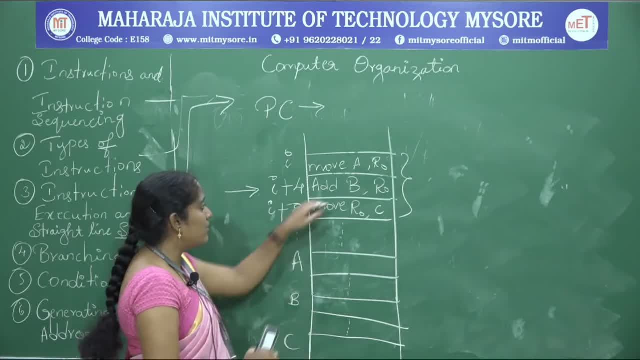 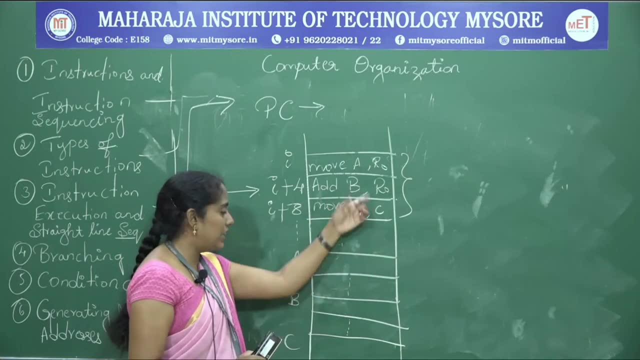 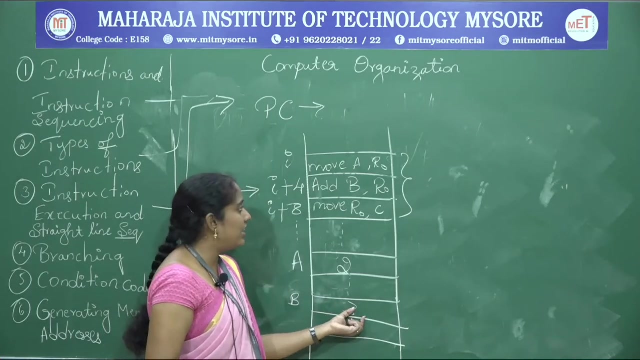 one by one, one after the other, right. So here also add is the instruction, move this, add instruction into the IR register and they take the content of B and search it here and take the content of B, say it is 2, 3.. So again, 3, add 3.. 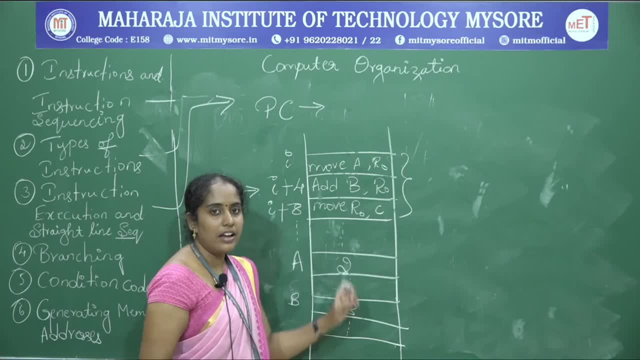 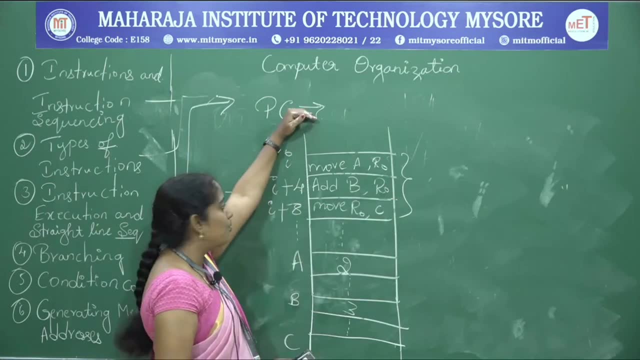 With the R0, contain value 2 and add 3 and 2, right, That is 5- and store the result in R0.. Again, again, the R. once this add instruction will move to the IR register, this PC value will be incremented. Now the PC value would contain the I plus 8.. So after the execution: 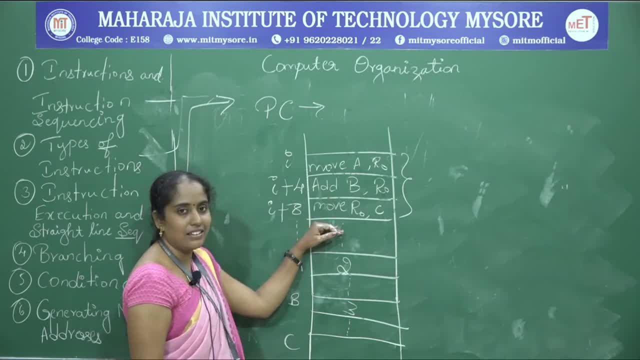 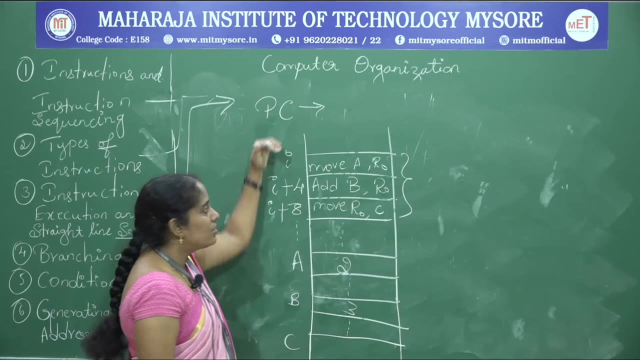 of this instruction, it will move to the next line. that is why it is called as straight line sequencing. So here, major work or the straight line sequencing, will be done by using this program counter. ok, So the next is. next topic is branching. So what do you mean by this branching? 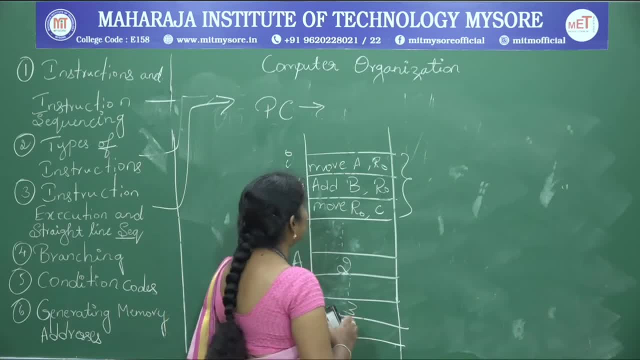 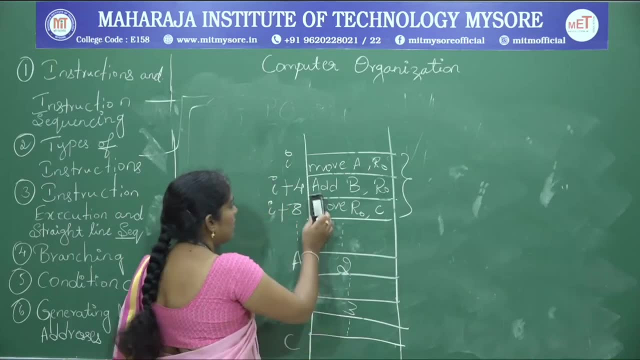 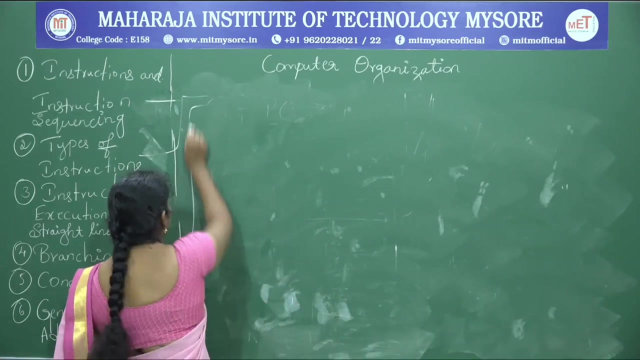 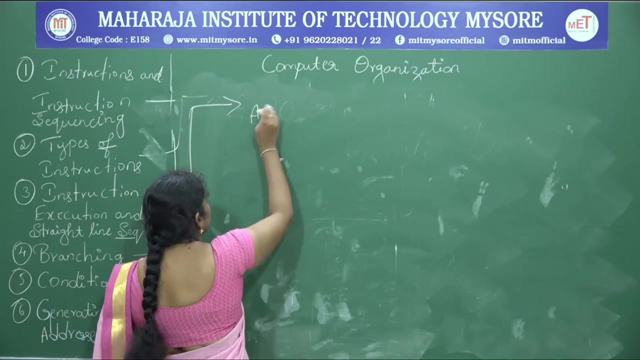 Take an example: addition of n numbers. How to write the addition of n numbers, How to write the instruction set for addition of n numbers. So for that, take an example: branching: addition of n numbers. So here, sum, right, Sum, ok, sum. 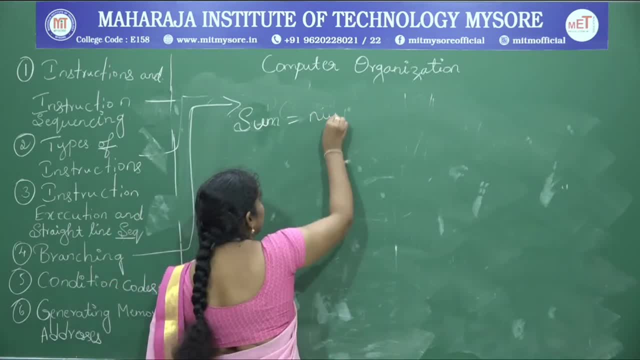 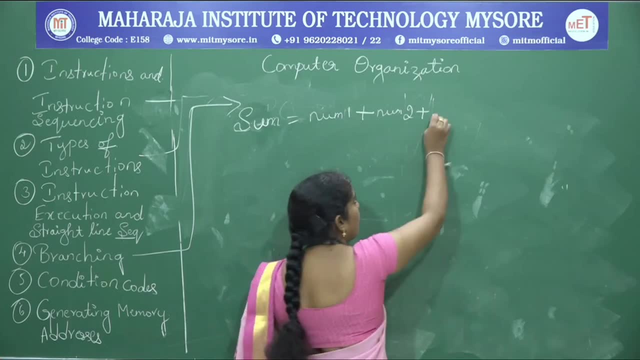 is equal to num1 plus, num2 plus and so on. num n: Ok, So this is the branching addition, ok So. sum Ok. So this is the branching addition of n numbers. So here, sum, Ok So. 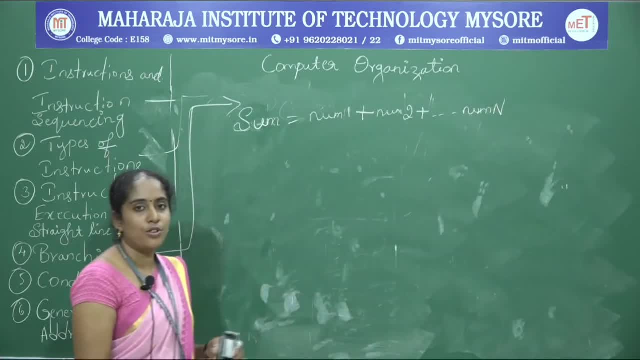 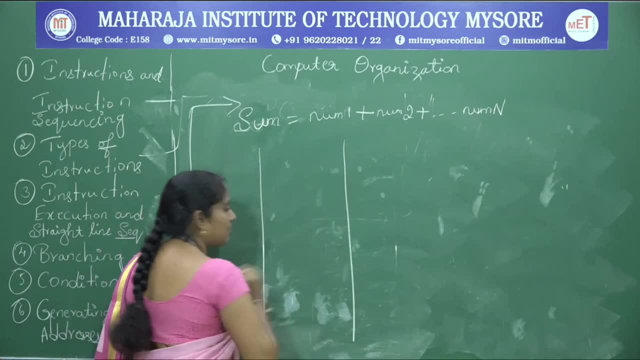 Right Here how to write this in the instruction. So for that, see for example: yes, this is your memory Right, This is the word Here. first move num1, r0.. num1, r0.. Next add num2, r0. Add num3, r0. Like that, Like that. 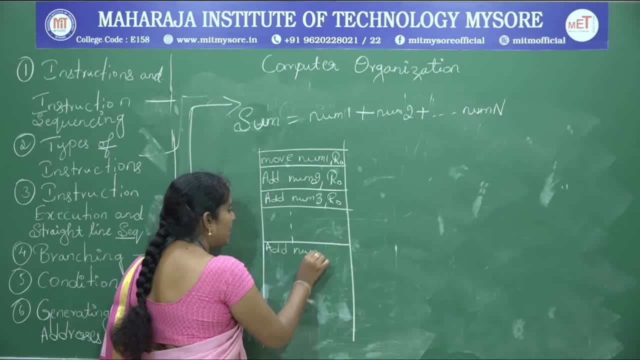 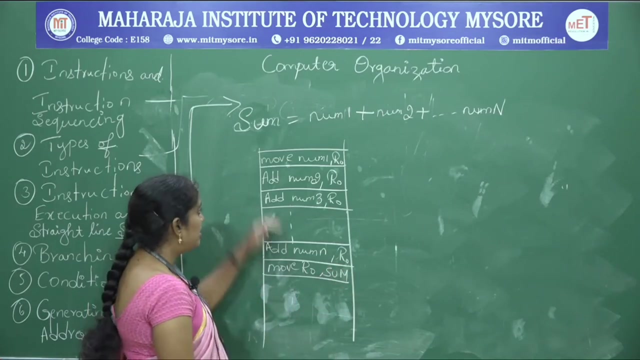 Add at last add. add num n r0. and the last one, which is that It is move num1, r0.. Move num2, r0.. r0. comma sum Right Here it takes more number of memory words. 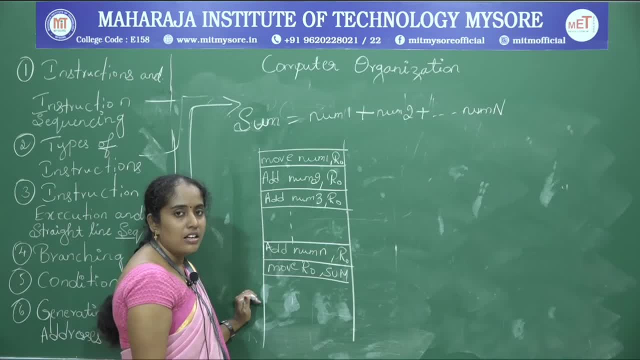 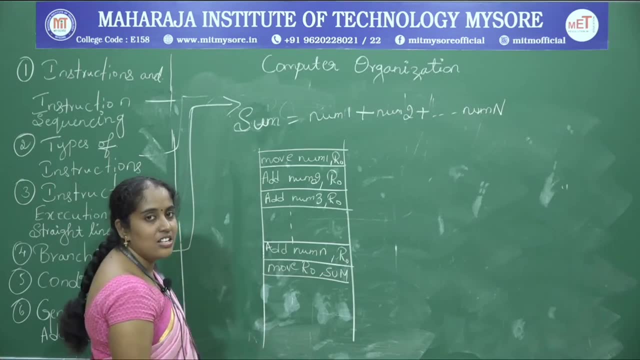 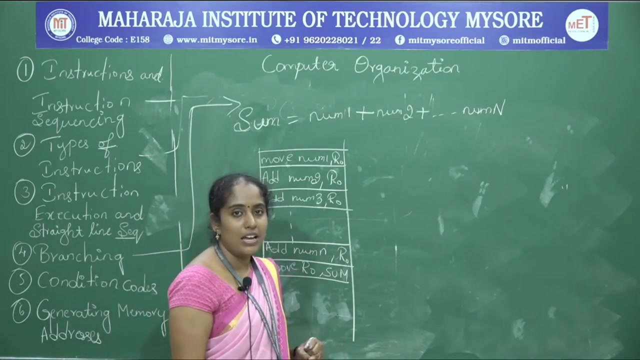 It occupies more words, Right. So to avoid this, to avoid this, we are using branching instructions Right, So branching instruction. So in the C programming language we are using while and for loop Right. Similar way, here also we are using 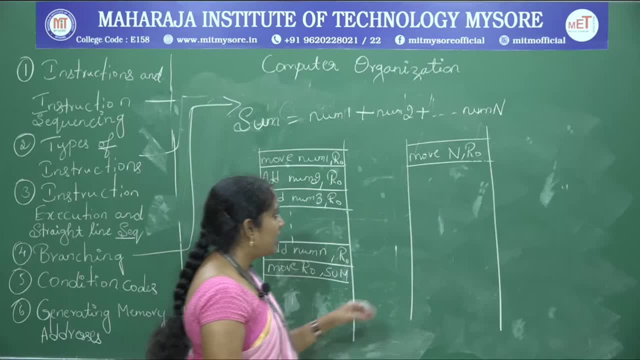 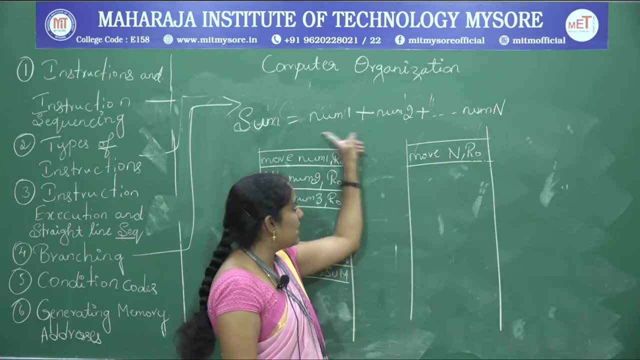 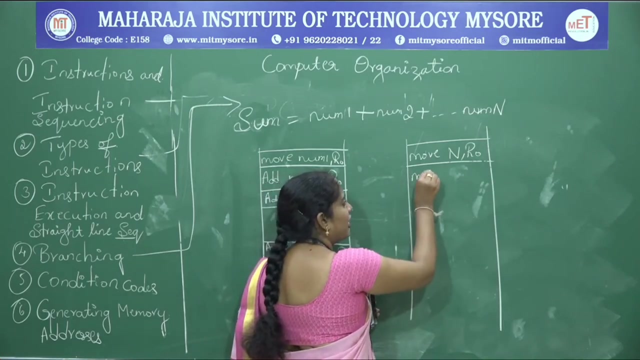 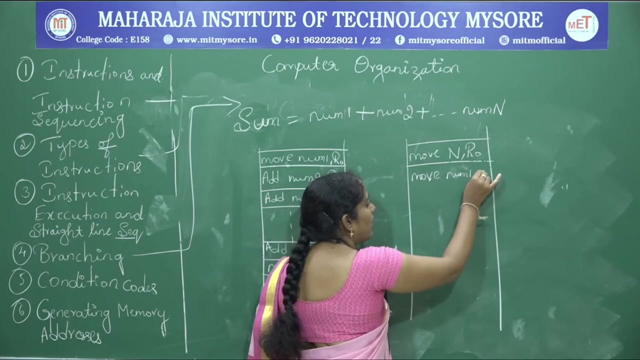 Similar way. here also we are using We are using branching instruction. Take an example: in the branching instruction First move n. n is the n numbers. This n numbers n value. That will be moved to r0.. Then then, first value, first value, num1 value will be moved to num1 comma, r1.. r1.. 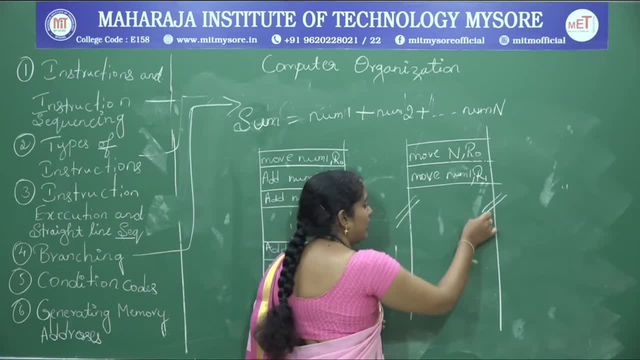 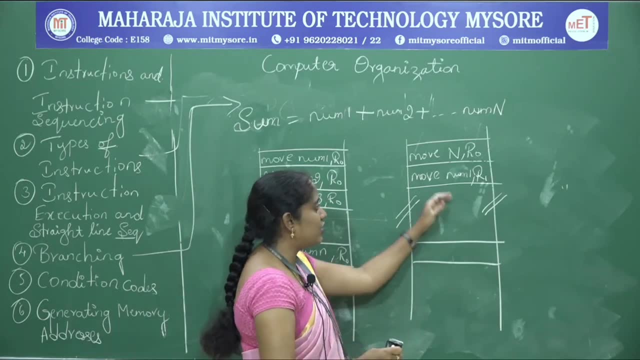 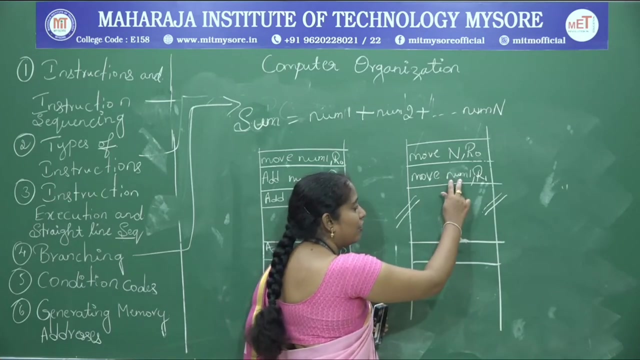 So after this we are using the, We are using the branching instruction or looping instructions. So after this here, So after the addition of first number with the num1.. Sorry, num1. addition of num1 with the num2.. So next you need to decrement. 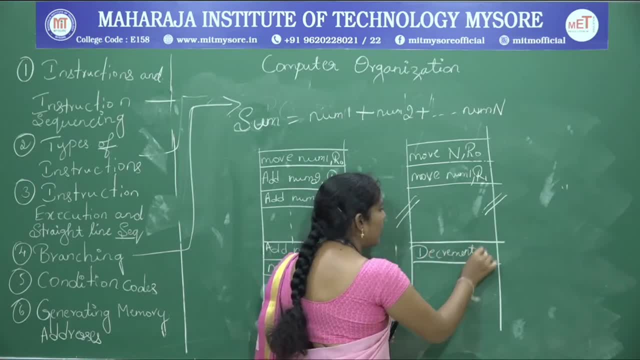 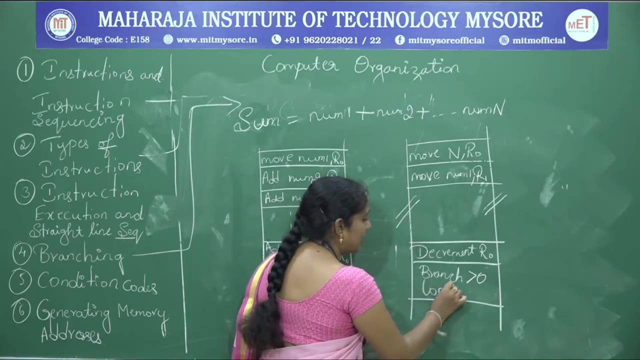 Here you need to decrement the r0 value. r0 value If the branch, If the here branch value is greater than 0. If this condition is true, Then go to the label. Particular label. That label name may be loop. 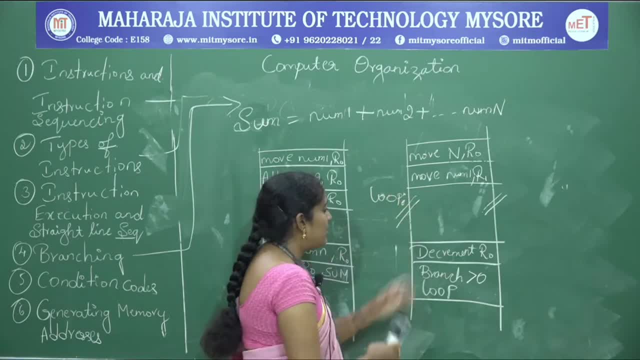 Here, this is the loop label, So this instruction will be executed n times, Right, This is called looping statement, So this can be anything. So here, what is this branch? This branch is nothing but this r0 value. So say, for example: 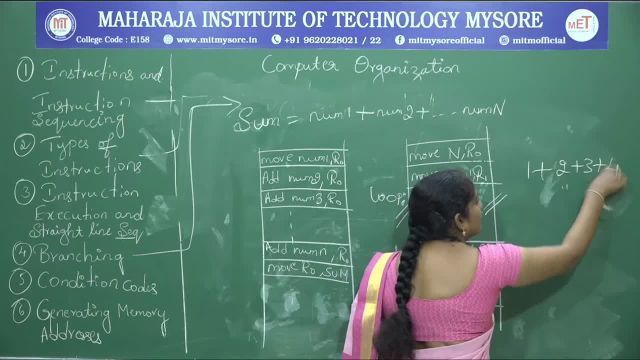 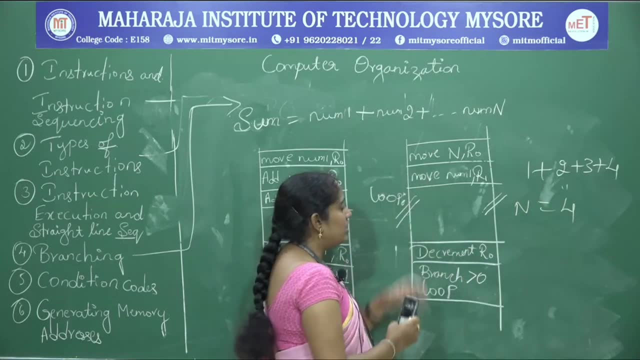 1 plus 2 plus 3 plus 4.. Right Here, what is the n value? n value will be 4.. n is 4.. Right, So initially r0.. You move r0.. n value to r0.. 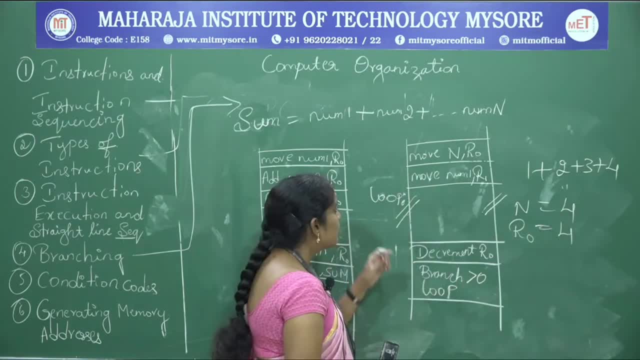 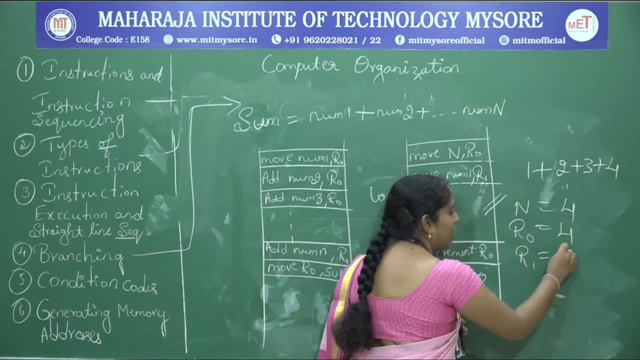 Then r0 also contain the value 4.. So now move num1.. What is the num1 value 1.. 1 will be moved to r1.. r1 will contain the value 1.. Right, So in this, In this, it will contain. 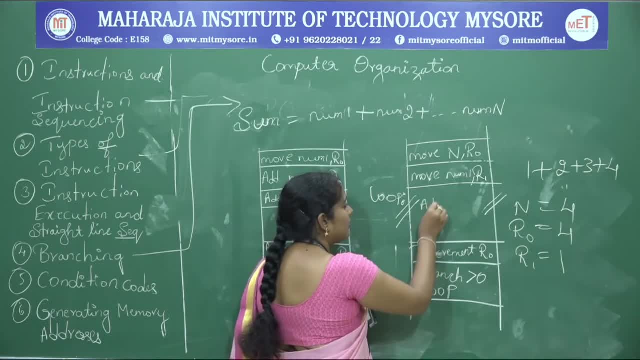 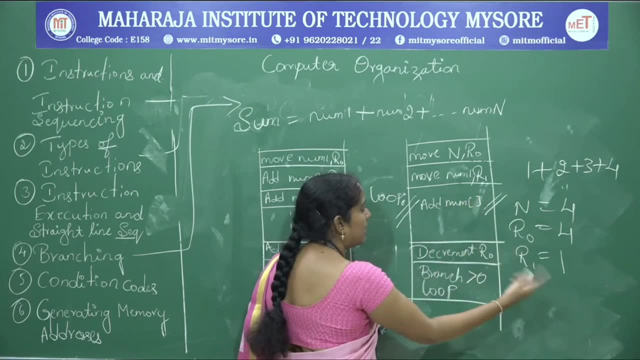 For example, Add num. We don't know the number Right num. Here it will incremented: Right, num2 comma r1.. Right, So num2.. What is the num2 value? It is 2.. Right 2 plus 1.. 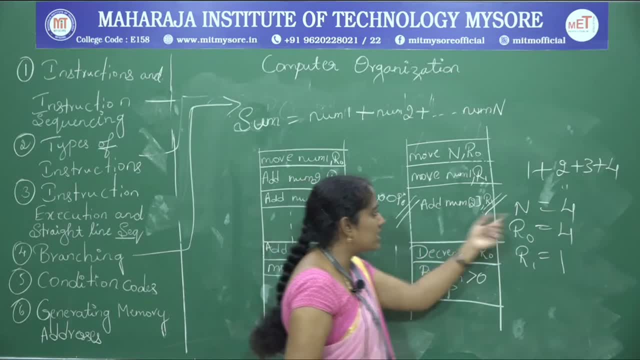 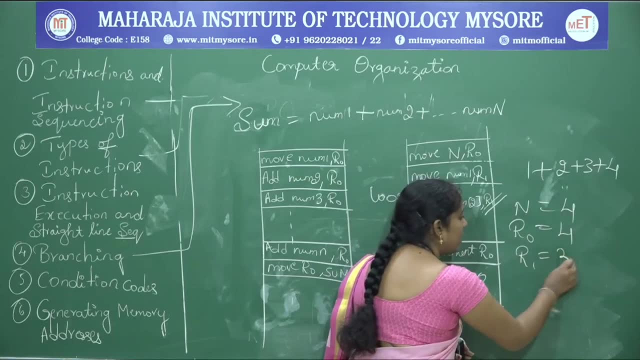 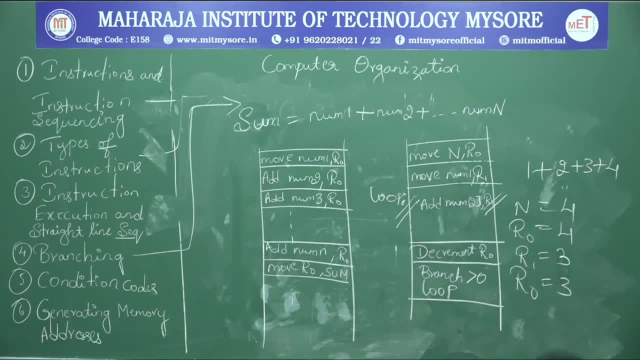 Now r0 will contain the value 3.. Right r0 will contain value 3.. Again check the condition. 3 is greater than 0.. Yes, Condition true. If the condition is true, Again, Go to the particular label. 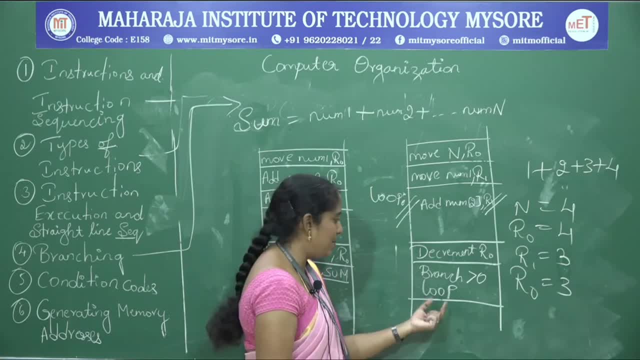 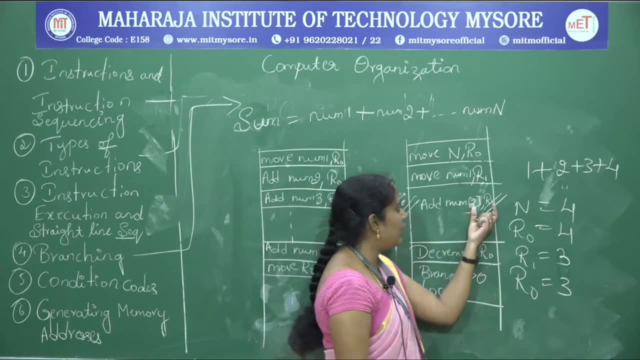 Label name is loop Again. Go back here And add Num 3. comma r1.. num 3. comma r1.. Here num3 value was 3.. 3 plus r1 value was 3.. 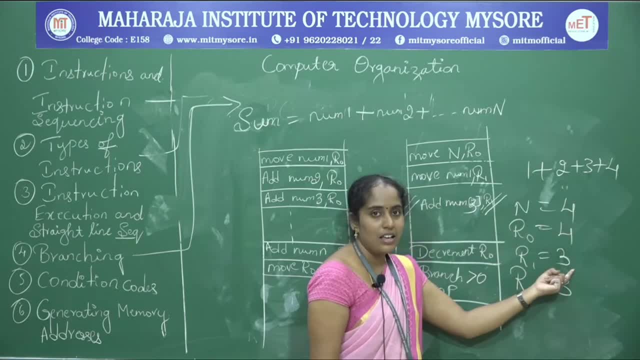 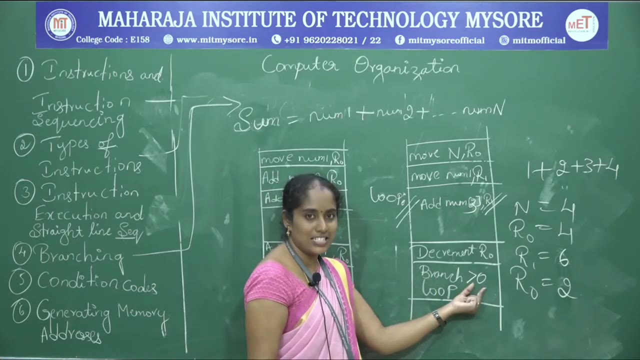 num2.. 3. comma: r1. value was 3.. Now R1 will contain the value 6.. Ok, Now decrement the R0 value. Now R0 value was 2.. Ok, So next is again check the condition. 2 is greater than 0.. Yes condition. 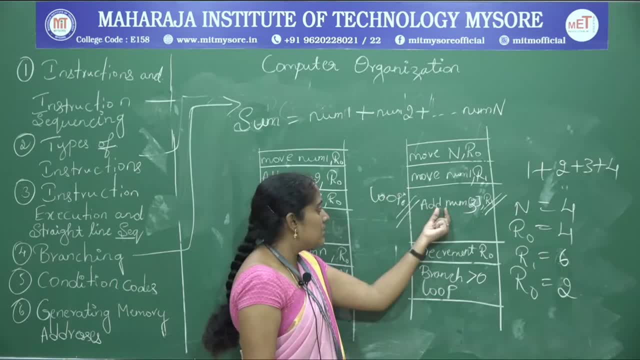 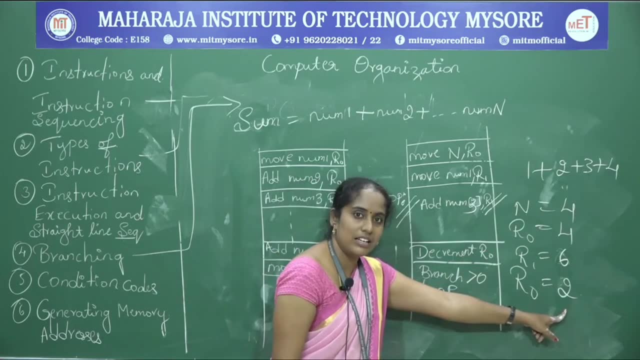 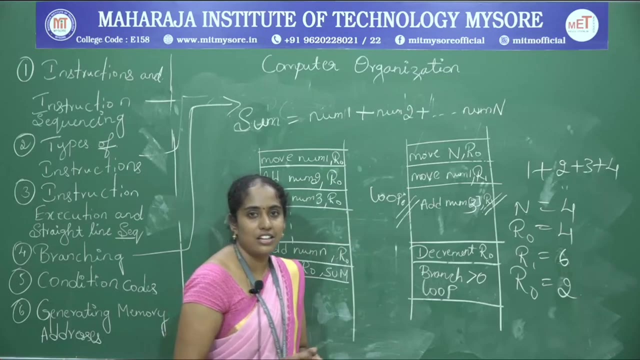 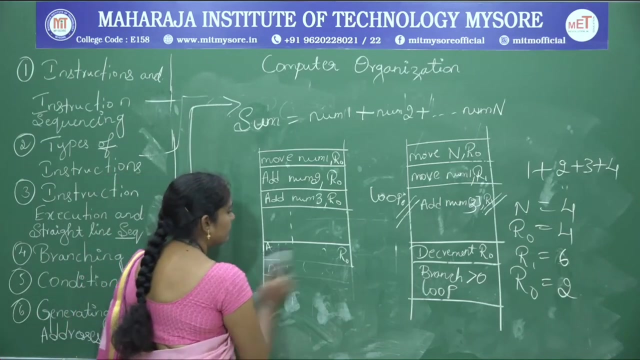 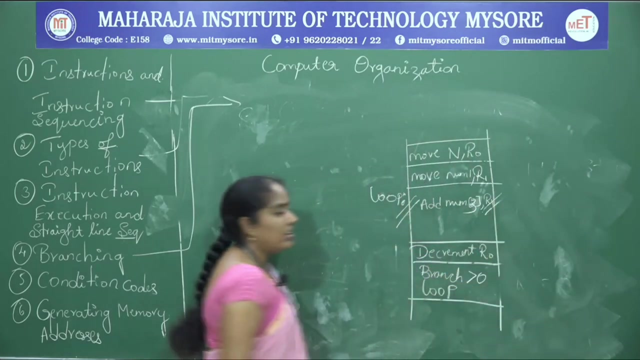 is true, So go to that particular label. So again, add num4 comma R1.. So now decrement the value R1.. Yes, it is decremented, and this will be repeated in n times. This is the branching instruction. Ok, So the next topic is conditional codes. Ok, What is this conditional code? 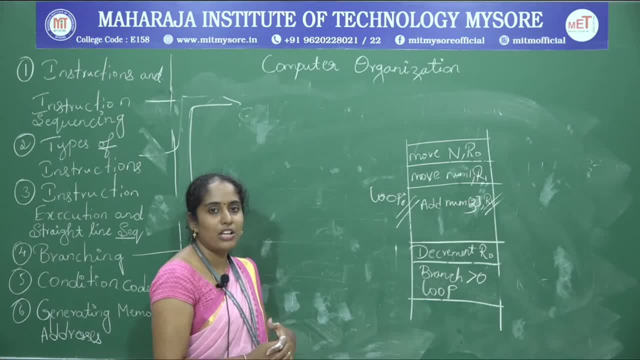 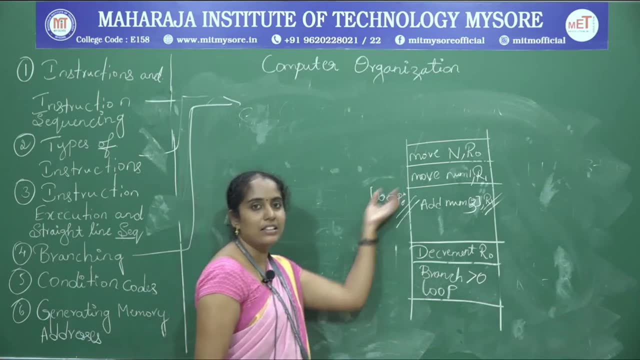 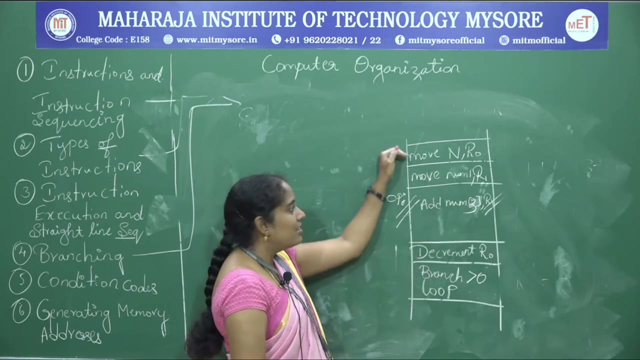 Here here, yes, as we know that program conditions Counter will contain the address of the next instruction to be executed, Right? So, in this example, in the conditional branching or conditional looping statements, in that case, Yes, Execute this, Execute this. Yes, It will contain the PC will contain the next instruction address. 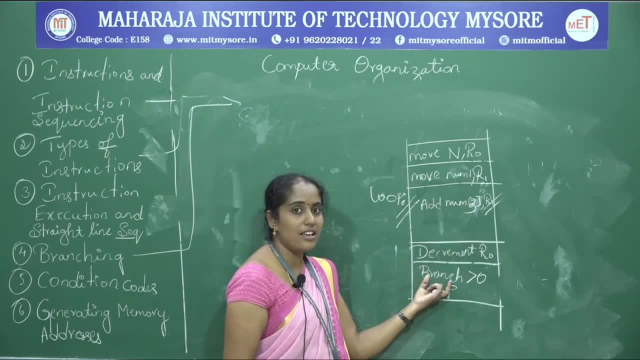 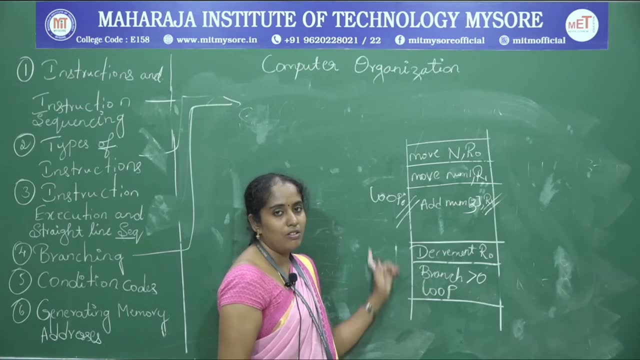 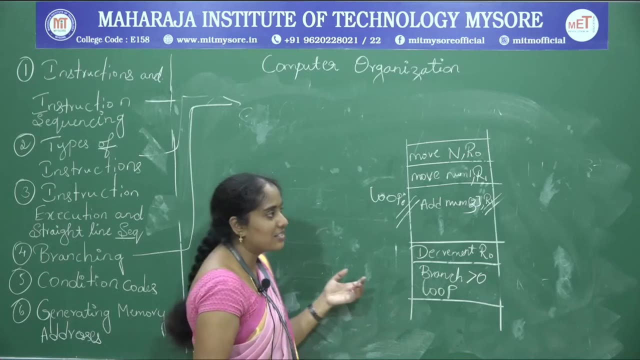 this one. So this one after this: if this condition is the condition is true, in that case, if the program counter value contain the next address, Then it will not be repeated in times. So for that reason we are using these flags, Conditional code flags. So conditional code flags is nothing but the flip flop. What is? 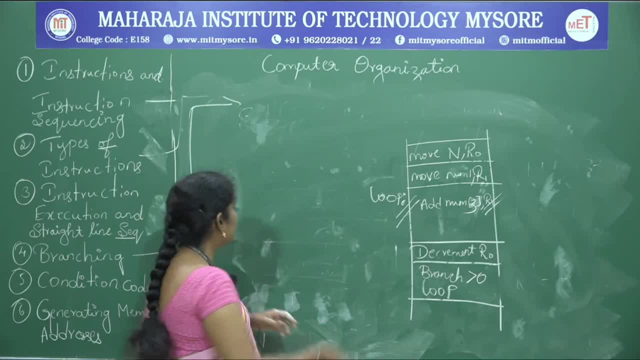 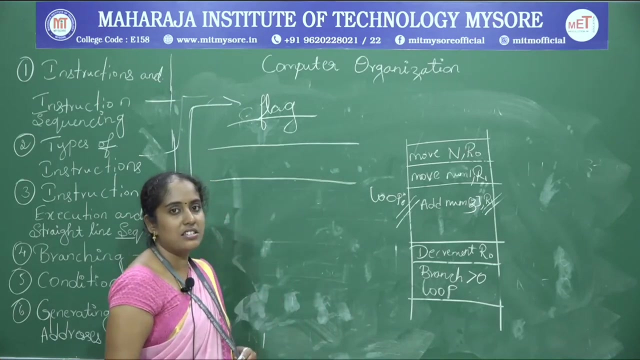 a flip flop, It is 0 or 1.. Right Say. for example, This is the conditional code Flag. conditional code: Flag is nothing but the resistor. OK, It is our special purpose register. This is the register memory location and it will contain four important conditional code. 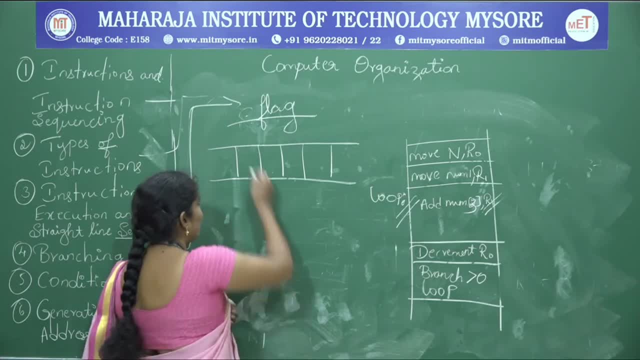 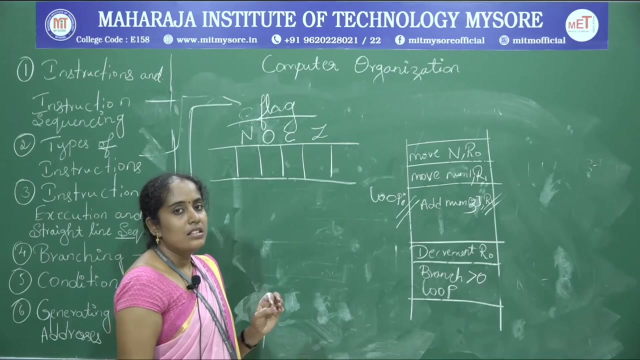 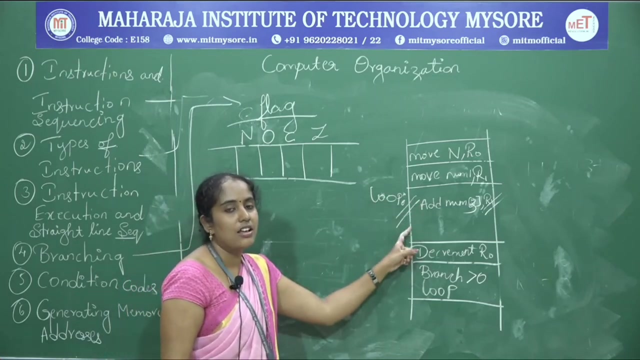 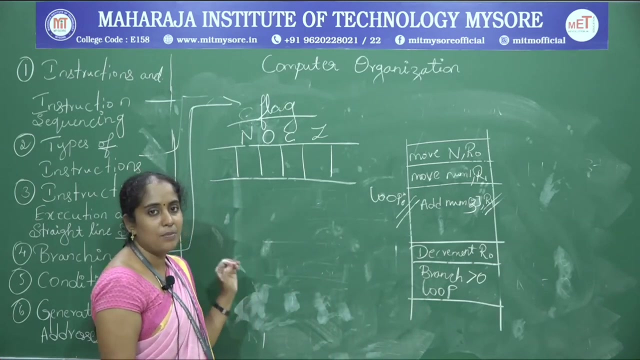 So that conditional code can be 0 or 1.. So in that first one is negative conditional code, overflow conditional code, carry conditional code and the 0 conditional code Say, for example, negative conditional code. So in this operation, in this looping operation, in the each step, in the each pass, if the result of any addition or subtraction value, if the result will be negative number, in that case set this n value to 1.. 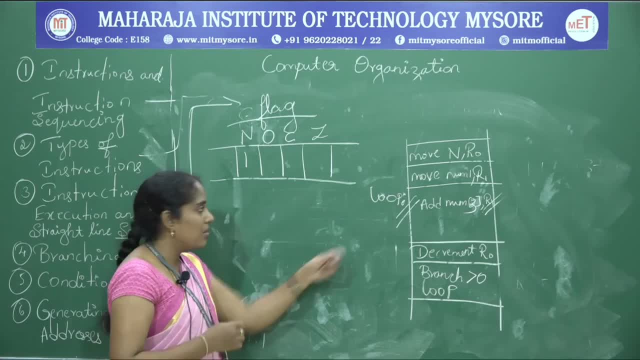 Or else if the result of that particular pass result will be positive, Positive number. in that case set this n value to 0.. So next is the O. O is the overflow condition. Say for example 1, 1.. Right. 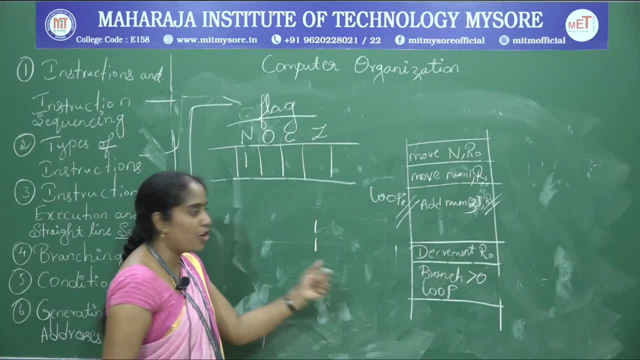 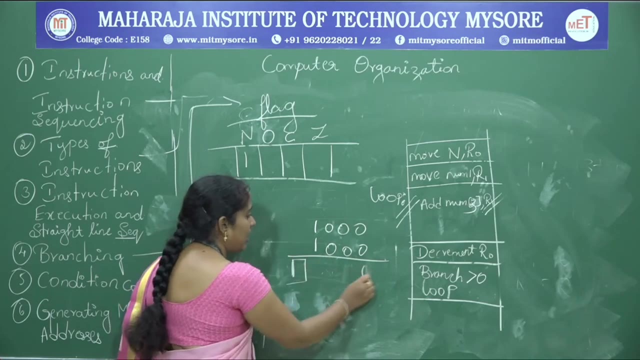 So in that case, say, for example, 4-bit addition In the 4-bit addition right, So the capacity of the register may be 4-bit. In that case the last one may be: see addition of this is: 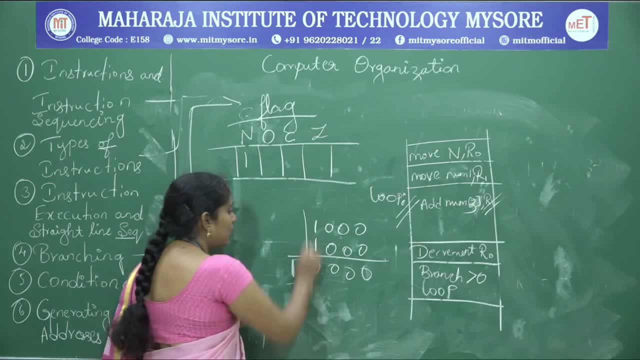 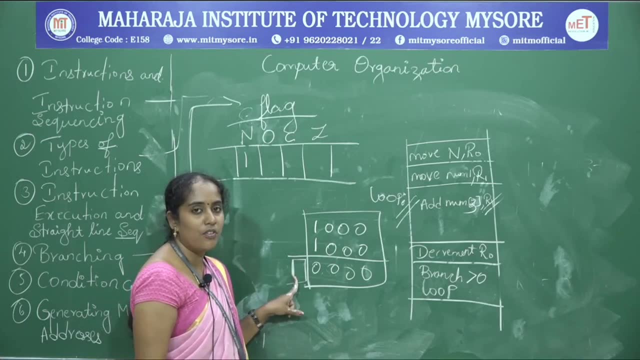 0 and carry 1.. So this is the overflow right, Because your register contain it can hold only 4-bits. In that case, this is overflow. How to identify the overflow? So in that case? so if the addition of these two numbers, it contains any one overflow, one value carry. 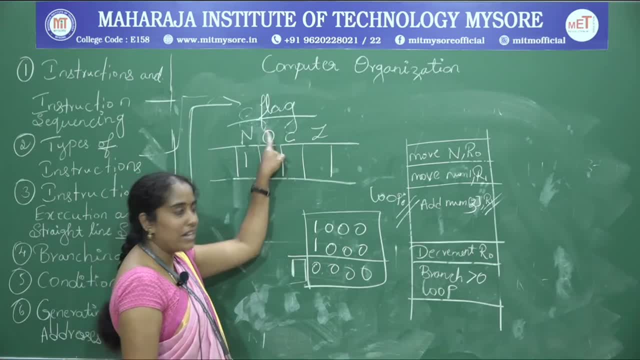 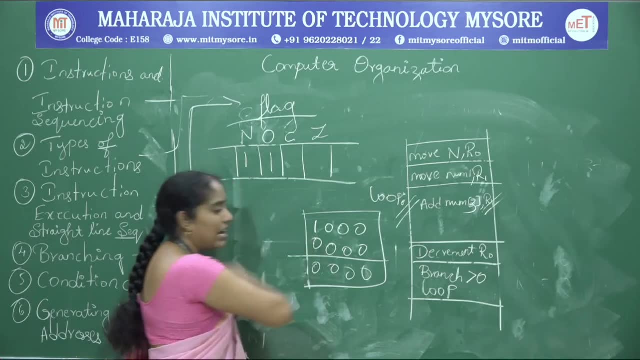 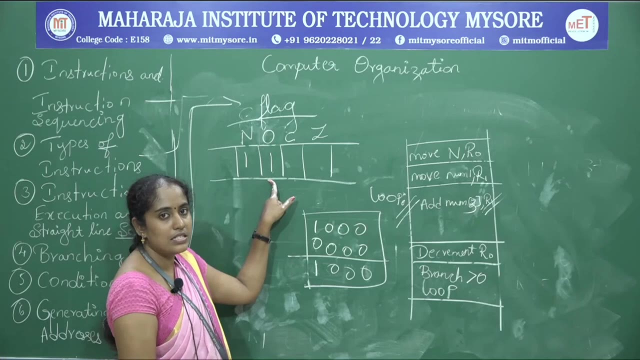 So in that case it will. this overflow bit will be set to 1. Say, if it is, it contains, say, for example, Addition of this number Here you cannot identify any overflow here, So in that case this bit will be set to 0.. 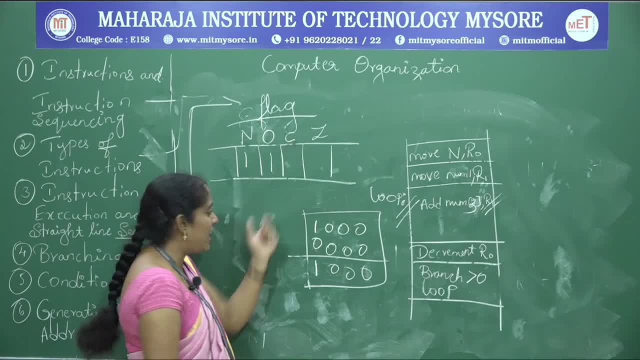 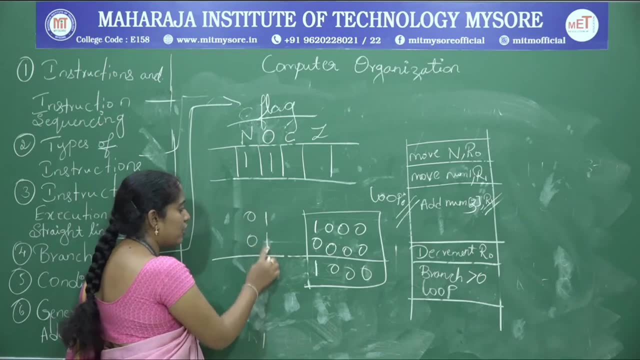 So next one is the carry flag. So carry flag say, for example, 1, 1,, 0, 0. So in that case 1, 1.. Right Addition of these two is 1,, 1 is 0 and carry 1.. 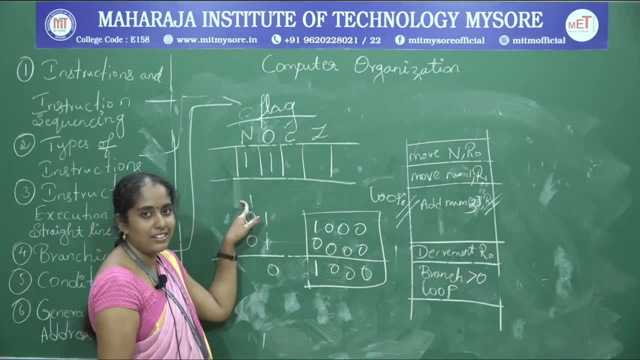 So in the next step, in the next loop, so this will be the carry right. How to identify this? In that case, the carry flag will be set to 0. Right, So in that case, it will be set to 1.. 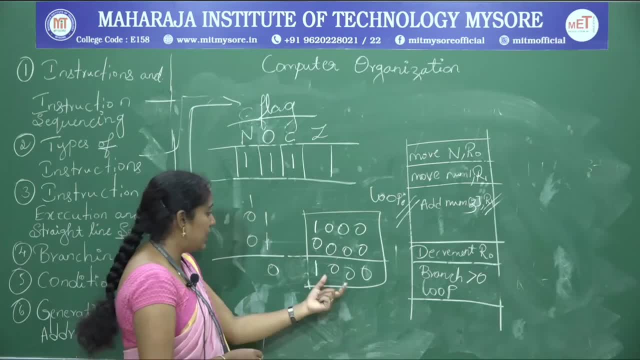 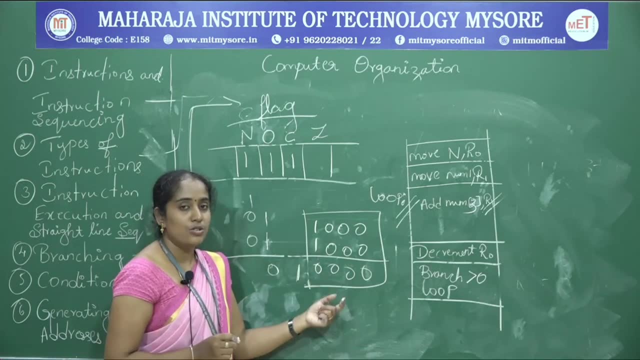 Right, Otherwise it will be set to 0.. So next is 0.. So in this, so in the previous example. So what is the answer for this? It is 0. Right, So in that case it will be set to if the answer of these two, addition of these two, will be 0. 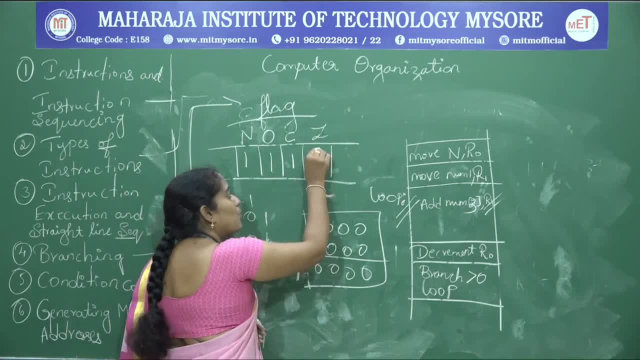 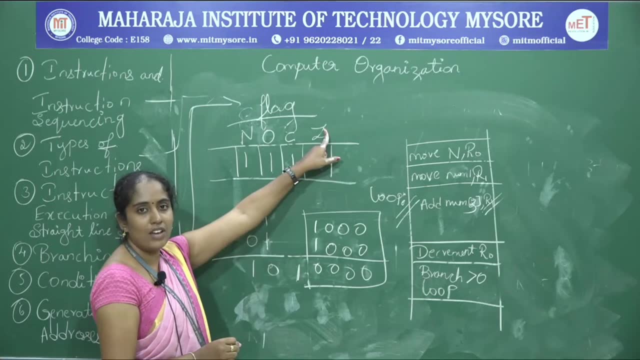 So in that case, this 0 flag will be set to set to 1, or else it will be set to 0. If any number. So in that in this case, This 0 flag will be set to 0..